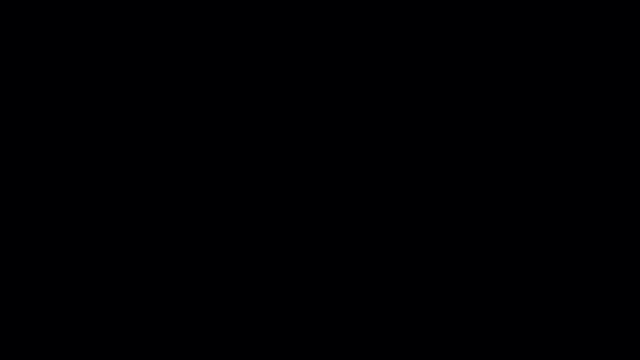 In this video, we're going to focus on mental math techniques. So, let's say if you want to add 34 plus 58 in your head. How would you do it? What's a quick and simple technique? So, what I like to do is I like to break down the numbers into small numbers. 34 is basically 30 plus 4. 58 is 50 plus 8. Now, it's pretty much straightforward to add 30 and 50. You know that 3 plus 5 is 8. So, 30 and 50 adds up to 80. And then 4 plus 8 is 12. 80 plus 12 is 92. 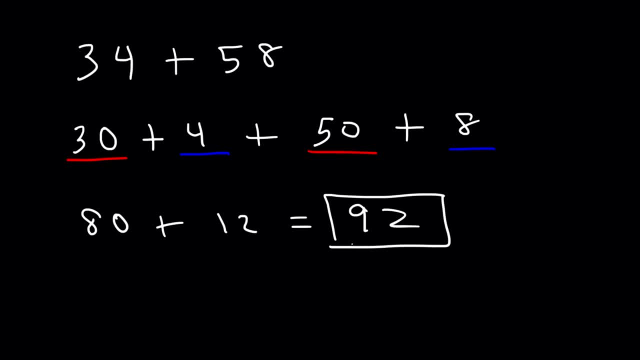 And so, that's a simple way to add two numbers. So, let's try another example. Go ahead and add 69 and 45. So, 69, we can write it as 60. 60 plus 9. 45 is 40 plus 5. Now, if we add 60 and 40, that's going to be 100. 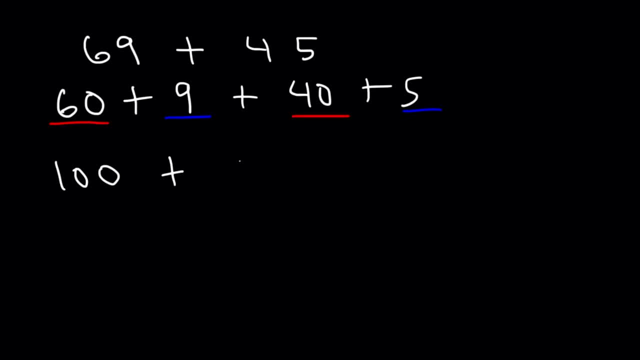 9 plus 5 is 14. 100 plus 14 is 114. Now, let's try some examples involving three-digit numbers. Go ahead and add 176 and 258. 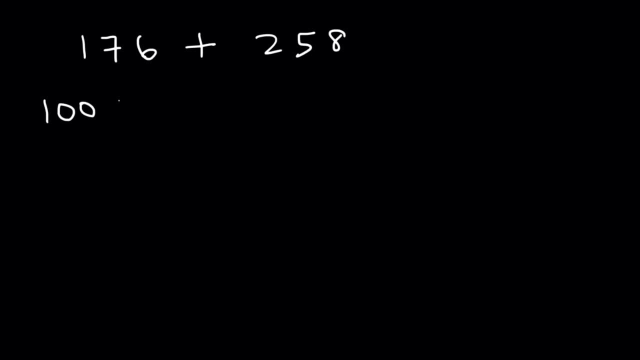 So, 176 is 100 plus 70 plus 6. 258 is 200 plus 50 plus 8. 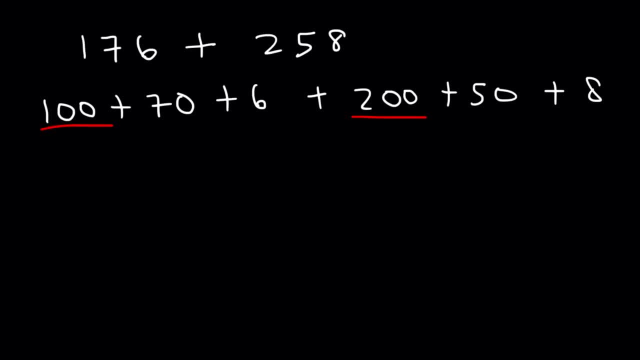 So, first, let's begin by adding 100 and 200. So, that's equal to 300. 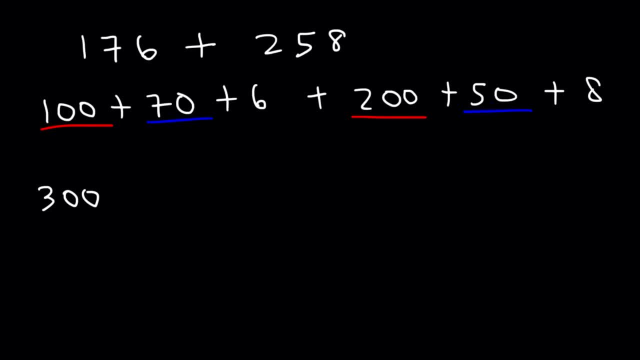 Now, if we add 70 and 50, how much is that? Well, we know that 7 plus 5 is 12. So, 70 plus 50 is 120. 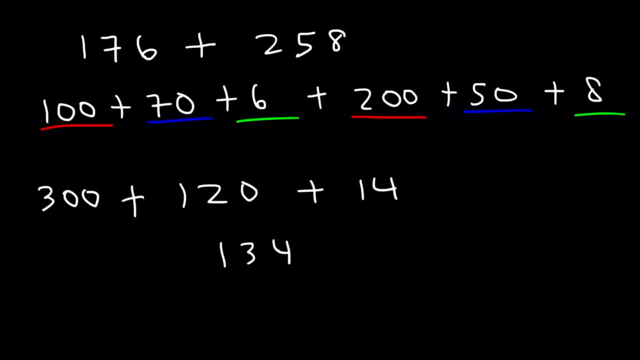 Now, 120 plus 14, that's 134. And if we add 300 to 134, it's 434. 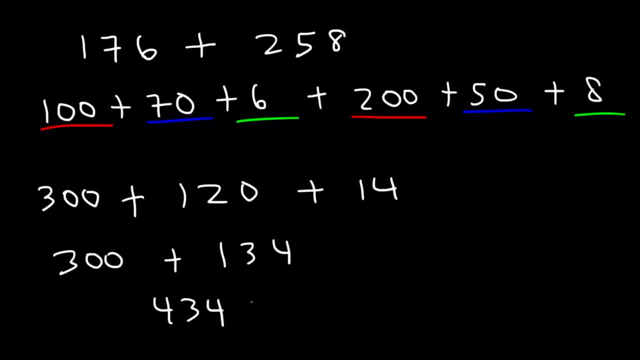 And if you have a calculator with you, you can add 176 plus 258. You should get 434. 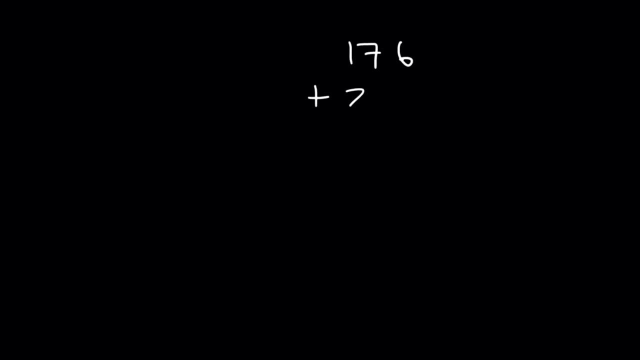 And of course, it's always good to review the old techniques. You can always add it by hand. 6 plus 8 is 14. Carry over the 1. 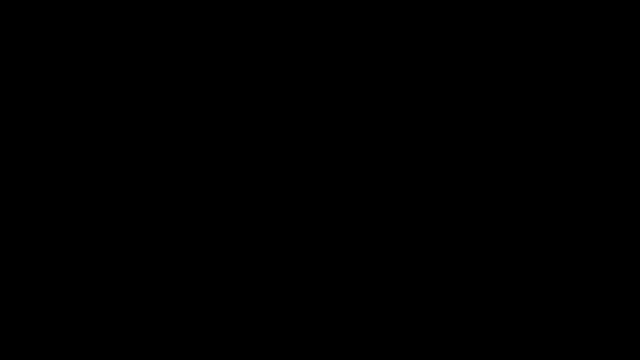 In this video we're going to focus on mental math techniques. So let's say, if you want to add 34 plus 58 in your head, How would you do it? What's a quick and simple technique. So what I like to do is I like to break down the numbers into small numbers. 34 is basically 30 plus 4.. 58 is 50 plus 8.. 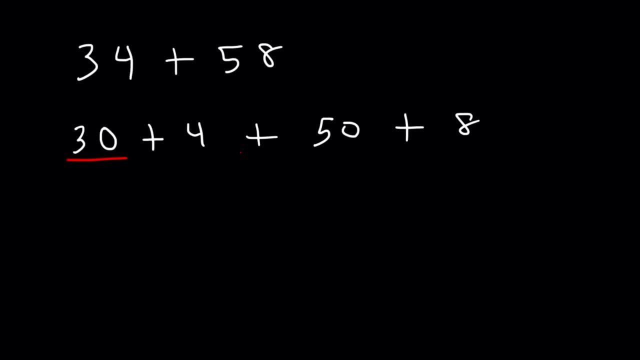 Now it's pretty much straightforward to add 30 and 50. You know that 3 plus 5 is 8. So 30 and 50 adds up to 80. And then 4 plus 8 is 12.. 80 plus 12 is 92.. 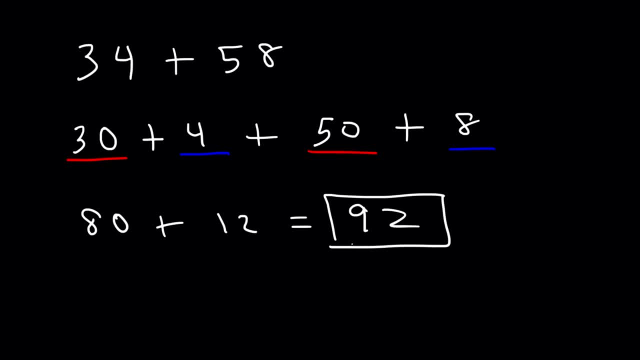 And so that's a simple way to add two numbers. So let's try another example. Go ahead and add 69 and 45.. So 69, we can write it as 60.. 60 plus 9.. 45 is 40 plus 5.. Now if we add 60 and 40, that's going to be 100. 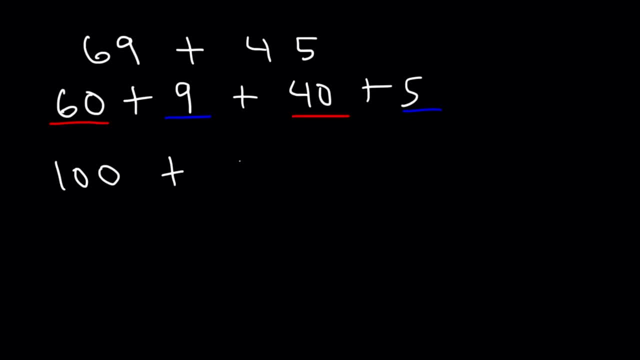 9 plus 5 is 14.. 100 plus 14 is 114.. Now let's try some examples involving three-digit numbers. Go ahead and add 176 and 258.. So 176 is 100 plus 70 plus 6.. 258 is 200 plus 50 plus 8.. 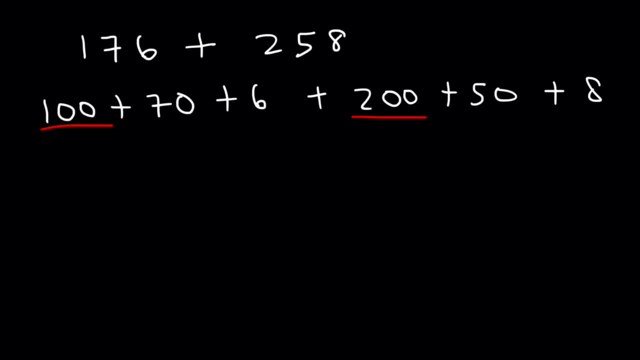 So first let's begin by adding 100 and 200.. So that's equal to 300.. Now, if we add 70 and 50, how much is that? Well, we know that 7 plus 5 is 12.. So 70 plus 50 is 120.. 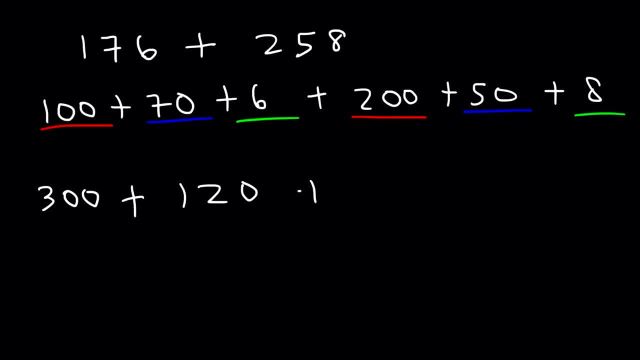 Now what about 6 plus 8?? 6 plus 8 is just 14.. Now, 120 plus 14, that's 134.. And if we add 300 to 134, it's 434.. And if you have a calculator with you, you can add 176 plus 258.. You should get 434.. 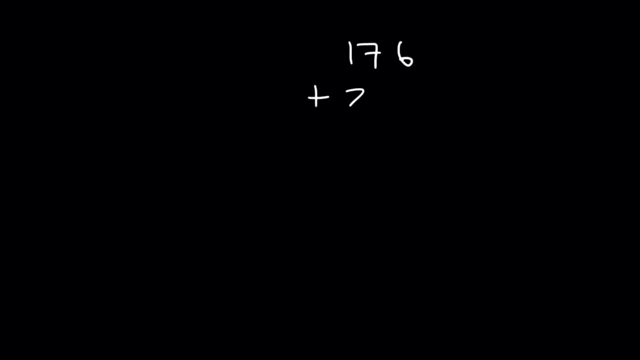 And of course it's always good to review the old techniques. You can always add it by hand. 6 plus 8 is 14.. Carry over the 1.. 1 plus 7 is 8 plus 5.. That's 13.. 1 plus 7 is 8 plus 5. That's 13. Carry over the other one. 1 plus 1 plus 2 is 4. So, you can confirm your answer using that method as well. 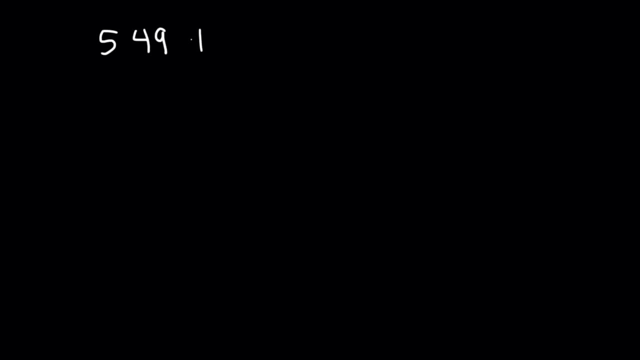 Here's another example. 549 plus 678. Feel free to pause the video and try that. 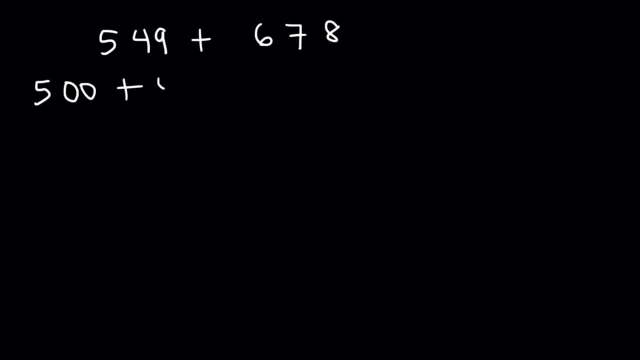 So, 549 is 500 plus 40 plus 9. 678 is 600. Plus 70 plus 8. 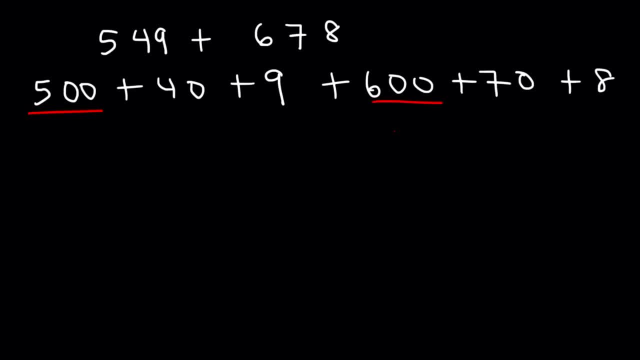 So, what's 500 plus 600? Well, we know 5 plus 6 is 11. So, 500 plus 600 is 1100 or 1100. 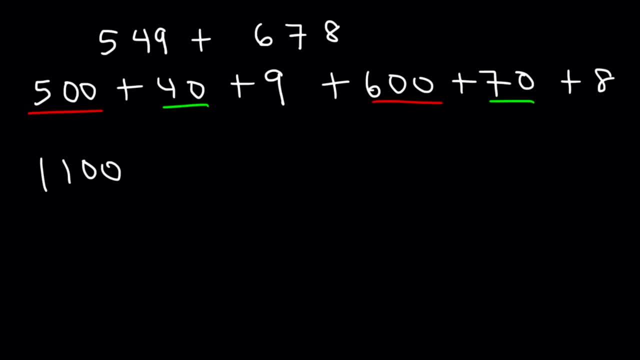 Now, what about 40 and 70? 4 plus 7 is 11. So, 40 and 70 is 110. 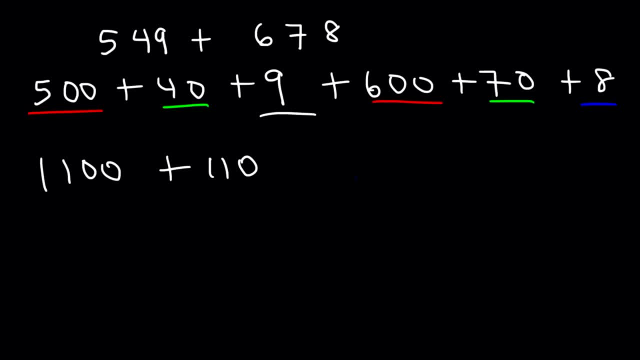 And then finally, we have 9 plus 8, which is 17. 110 plus 17 is 127. And if you add 127 to 100, that's 227. 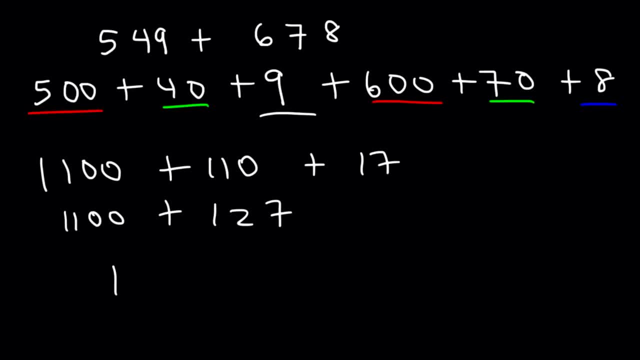 So, 1100 plus 127 must be 1227. And so, that's the final answer. 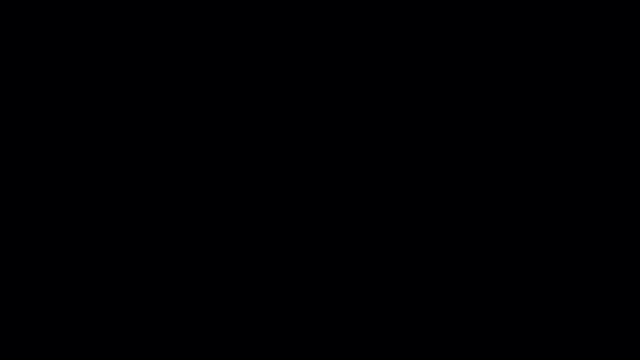 Now, let's try some examples involving subtraction. What is 75 minus 38? So, we can use the same technique. We can break down 75 into 70 plus 5. And 38 is basically 30 and 8. But you need to apply the negative sign to both numbers. Not just the 30. Otherwise, it's not going to work. 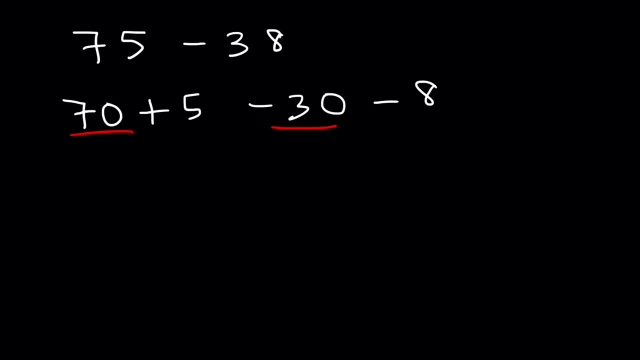 So, now, 70 minus 30, that's equal to 40. So, we have 40 plus 5 minus 8. Now, 5 minus 8 is a negative number. That's going to be 9. That's going to be negative 3. And 40 minus 3 is 37. So, 37 is your final answer. 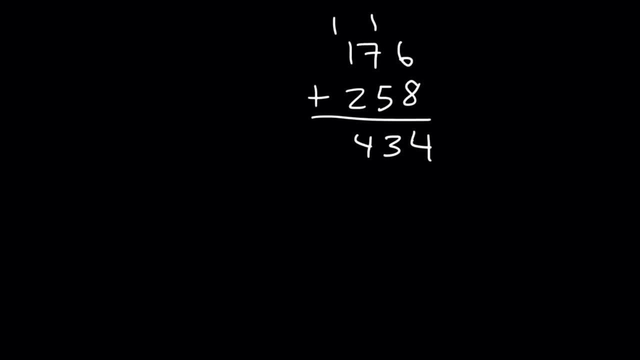 Carry over the other one. 1 plus 1 plus 2 is 4.. So you can confirm your answer using that method as well. Here's another example: 549 plus 678.. Feel free to pause the video and try that. 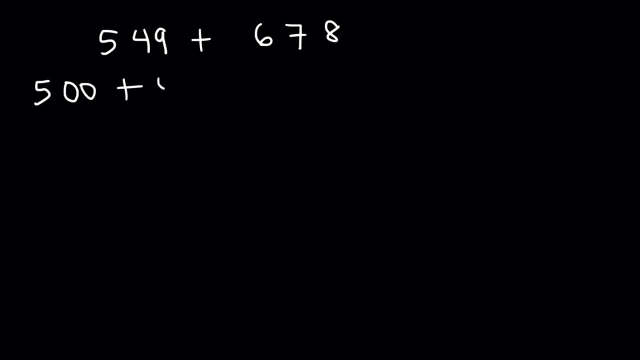 So 549 is 500 plus 40 plus 9.. 678 is 600.. Plus 70 plus 8. So what's 500 plus 600?? Well we know, 5 plus 6 is 11.. So 500 plus 600 is 1100 or 1100.. 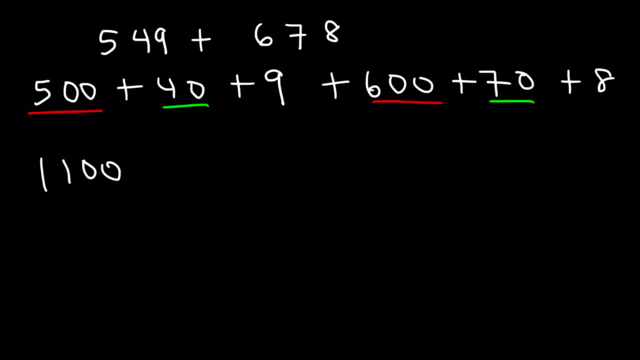 Now what about 40 and 70?? 4 plus 7 is 11.. So 40 and 70 is 110.. And then, finally, we have 9 plus 8,, which is 17.. 110 plus 17 is 127.. 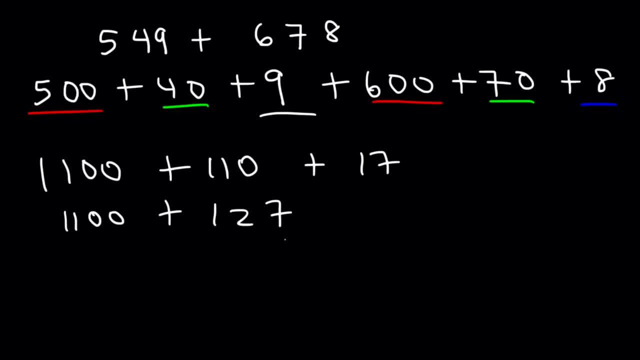 And if you add 127 to 100, that's 227.. So 1100 plus 127 must be 1227.. And so that's the final answer. Now let's try some examples involving subtraction. What is 75 minus 38?? 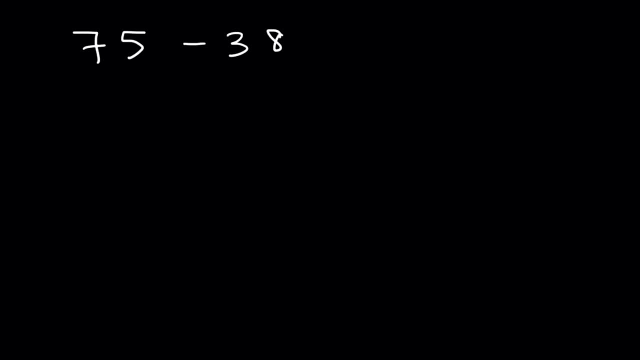 So we can use the same technique. We can break down 75 into 70 plus 5. And 38 is basically 30 and 8. But you need to apply the negative sign to both numbers, Not just the 30.. 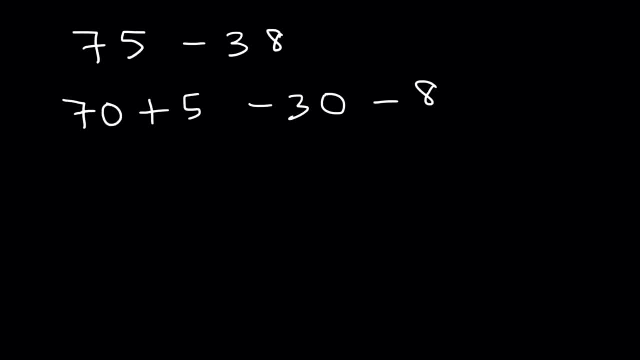 Otherwise it's not going to work. So now, 70 minus 30, that's equal to 40. So we have 40 plus 5 minus 8. Now 5 minus 8 is a negative number. 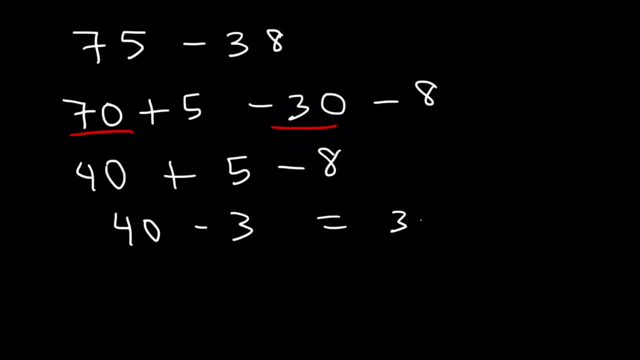 That's going to be 9.. That's going to be negative 3.. And 40 minus 3 is 37. So 37 is your final answer. Now, what about this? 143 minus 56.. Go ahead and work on that example. 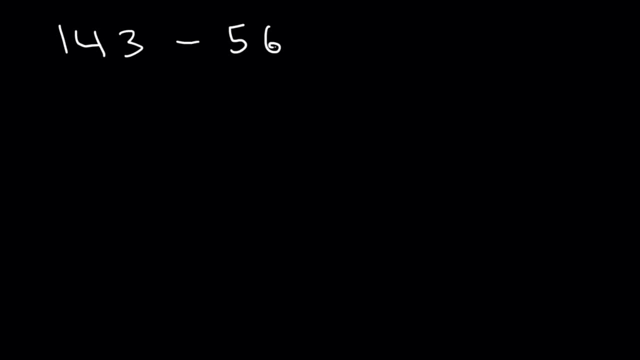 Now what about this? 143 minus 56. 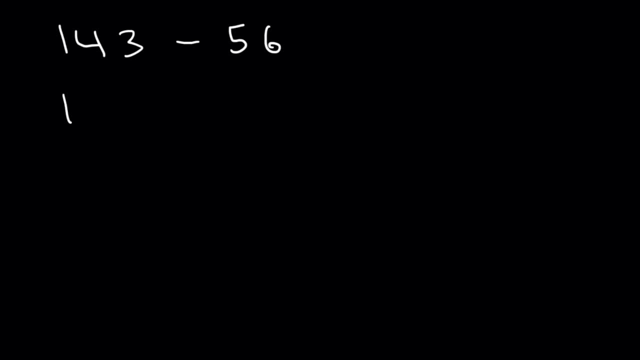 Go ahead and work on that example. So, we can write this as 100 plus 40 plus 3. And 56, we can write that as 50 and 6, making both numbers negative. Now. And then, 100 minus 10. That's 3 and 6. So, you just get 1, 2, 3, 6, 6. 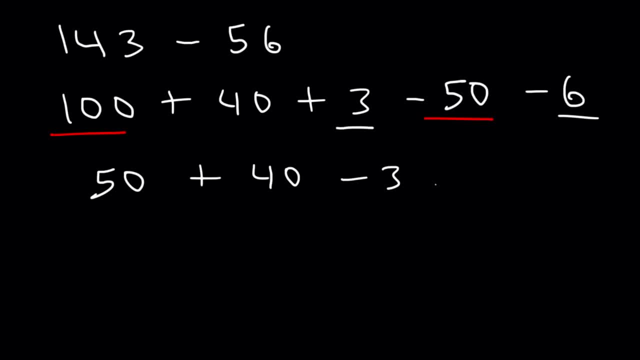 So, 1 to the power of 30 minus 30 and 7. That's 3. That's 3. That's 1. So, let's doètex. 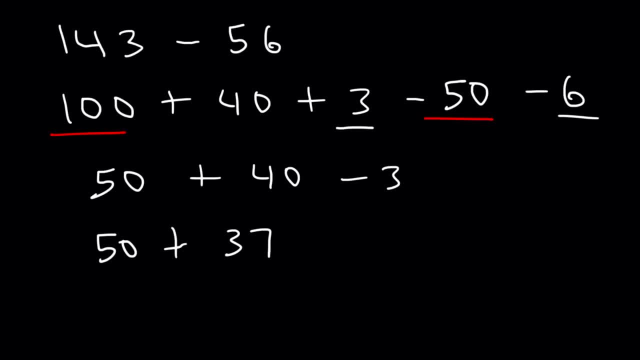 1 to the. three is 37 and 80 plus 37 I mean 50 plus 37 is 87 so that's going to be your 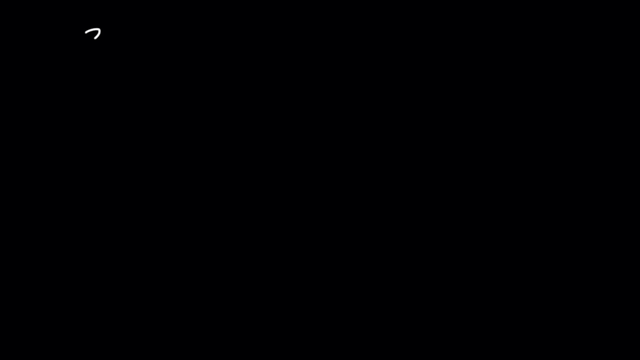 answer for this example let's work on an example with three digit numbers try that so let's break down 356 into 300 plus 50 plus 6 and negative 189 is going to be minus 100 minus 80 minus 9 so let's start with 300 minus 100 3 minus 1 is 2 so 300 minus 100 is 200 next we have 50 minus 80 which is negative 30 since 5 minus 8 is negative 3 and then we have 6 minus 9 which is negative 3 now 200 minus minus 30 that is equal to a hundred and seventy and 170 minus 3 that's going to be 167 and so that should be the final answer now you can confirm it by subtracting these numbers by hand now 6 minus 9 we can't subtract it's a negative number so we need to borrow a 1 from the 5 so that's going to turn into 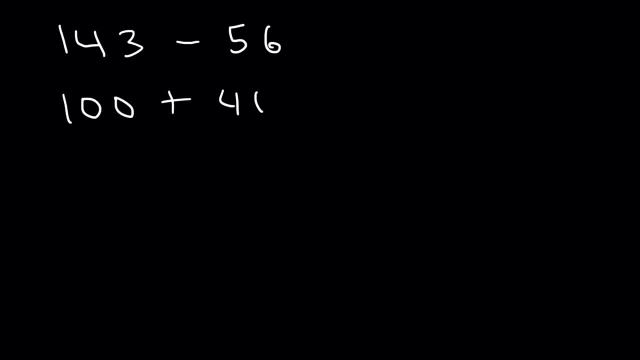 So we can write this as 100 plus 40 plus 3.. And 56, we can write that as 50 and 6, making both numbers negative Now. So we have 100 minus 50.. So we can write this as 50 plus 50.. 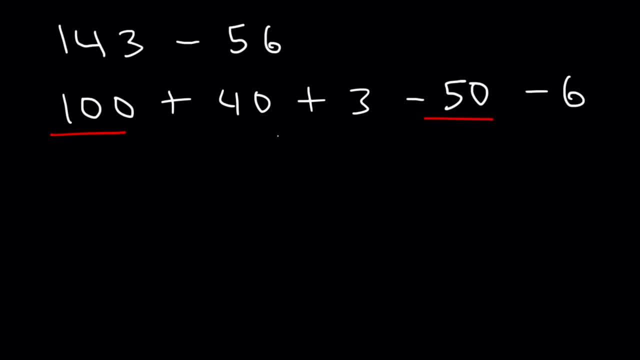 And we can write this as 100 minus 50. There's many ways in which you can do this, But let's do 100 minus 50, because that's positive 50. And 3 minus 6. Well, that's going to be negative 3.. 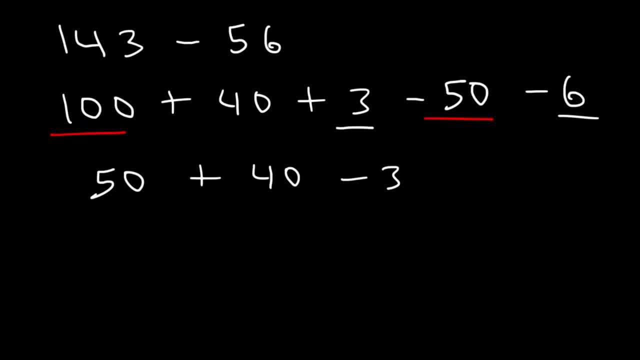 You can do this in many different orders. So you just pick and choose whichever order you feel comfortable in doing this. Now, 40 minus 3. That's going to be negative 3. So you just pick and choose whichever order you feel comfortable in doing this. 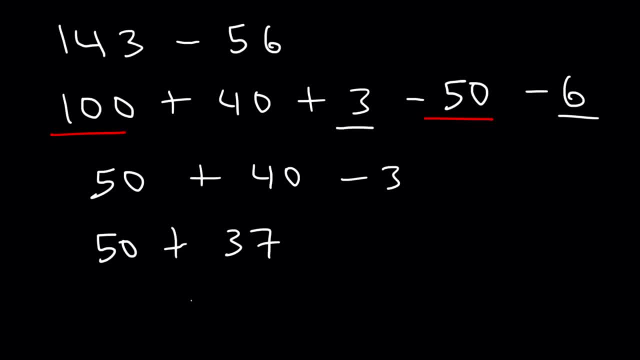 37 and 80 plus 37- I mean 50 plus 37- is 87, so that's going to be your answer for this example. let's work on an example with three digit numbers. try that. so let's break down 356 into 300 plus 50 plus 6, and negative 189 is going to be. 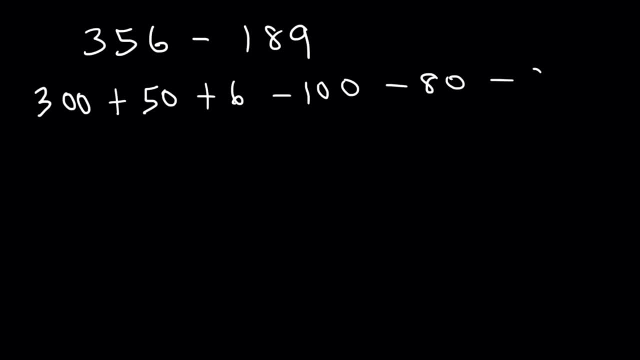 minus 100 minus 80 minus 9, so let's start with 300 minus 100. 3 minus 1 is 2, so 300 minus 100 is 200. next we have 50 minus 80, which is negative 30, since 5. 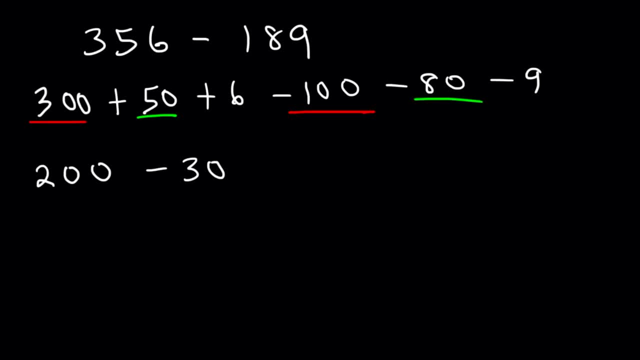 minus 8 is negative 3. and then we have 6 minus 9, which is negative 3. now 200 minus 8 is negative 3, so that's going to be negative. 6 minus 9 is negative 3, so that's 30, that is equal to 170.. And 170 minus 3, that's going to be 167. And so that should be the final. 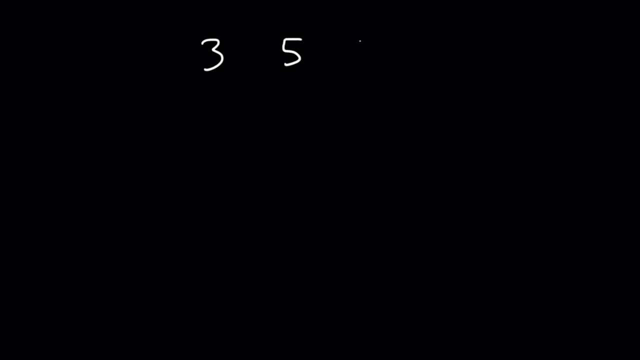 answer Now. you can confirm it by subtracting these numbers by hand. Now, 6 minus 9, we can't subtract it. It's a negative number, So we need to borrow a 1 from the 5.. So that's going to turn. 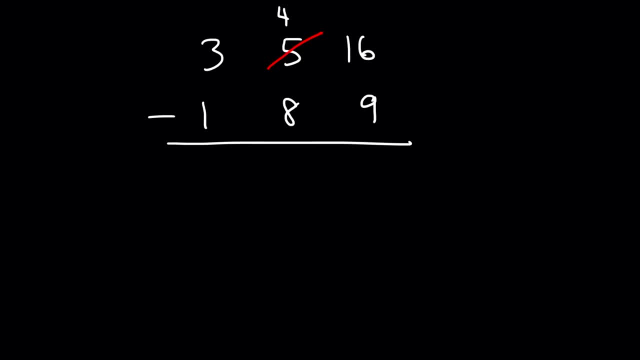 into a 4.. We're going to carry over a 1 to the 6, making it 16.. 16 minus 9 is 7.. Now 4 minus 8 is a negative number, So we're going to have to borrow another 1, making this 2 and making the 4. 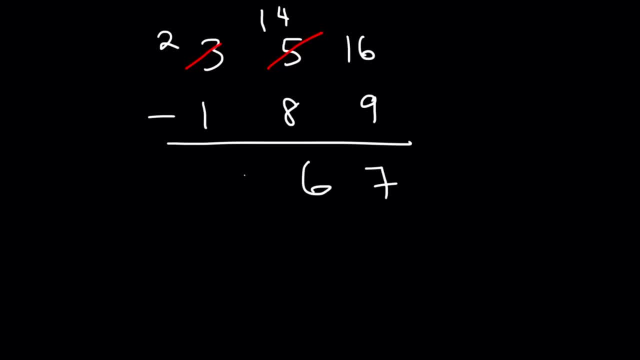 14.. 14 minus 8 is 6.. 2 minus 1, 1.. So we get 167.. So you can confirm it using that technique. Now let's work on simple multiplication problems. What is 5 times 4?? So hopefully you've committed this to memory, You. 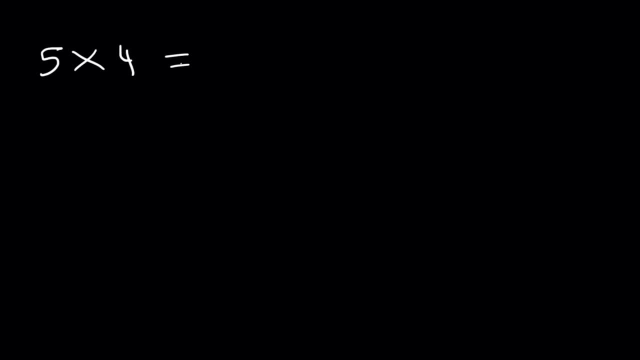 know your multiplication tables up to 12.. But let's say, if you don't know it, What is 5 times 4?? 5 times 4 is basically 5 added 4 times Multiplication. what it really is is repeat. 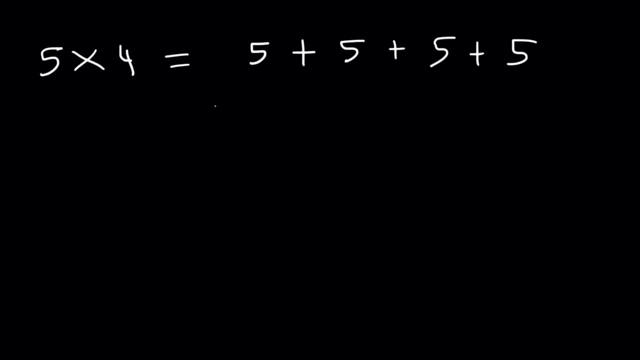 addition. So 5 times 4 means you're adding 5. 4 times 5 plus 5 is 10.. The other two 5s add up to 10.. 10 plus 10 is 20.. So 5 times 4 is 20.. You. 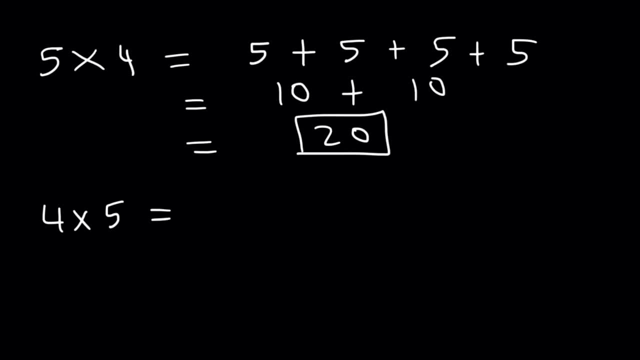 could also see it this way: 5 times 4 and 4 times 5 are the same. 4 times 5 means that you're adding 4. 5 times 4 plus 4 is 8.. The next two 4s add up to 8.. And then we have one 4 remaining. 8 plus 8 is 16.. 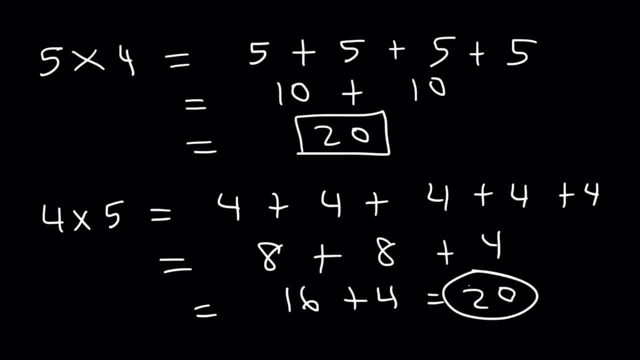 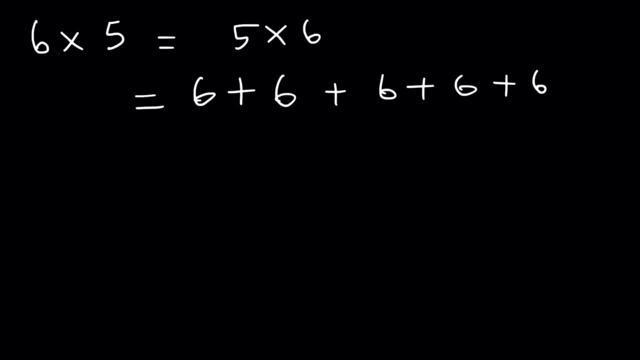 16 plus 4 is 20.. So you get the same answer. So let's say, if we want to find the value of 6 times 5, which is the same as 5 times 6.- All we need to do is add 6- 5 times, or add 5- 6 times, whichever. 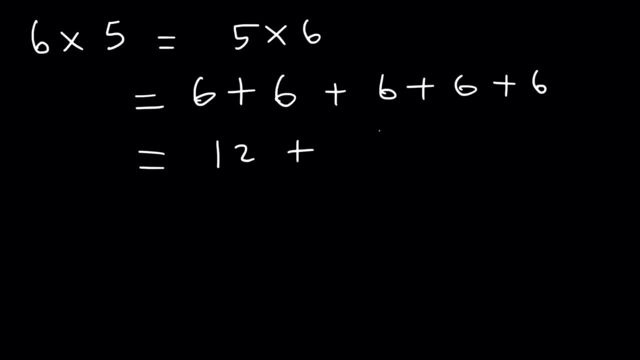 is easier: 6 plus 6 is 12,, so these two add up to 12 as well, And 12 plus 12 is 24, plus 6,, that's 30. So 6 times 5, or 5 times 6, is 30. Now what about 8 times 3?? This is simply 8 plus 8 plus 8. 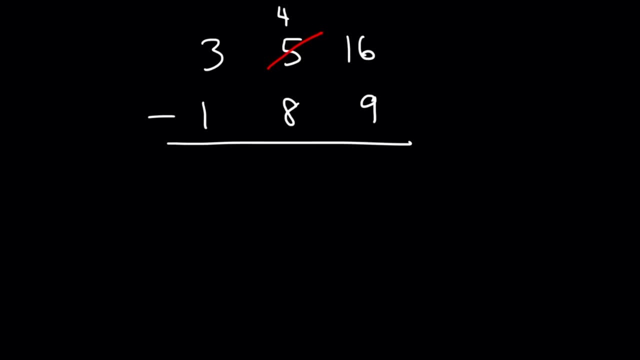 a 4 we're going to carry over 1 to the 6 making it 16 16 minus 9 is 7 now 4 minus 8 is a negative number so we're going to have to borrow another one making this 2 and making the 4 14 14 minus 8 is 6 2 minus 1 1 so we get 167 so you can 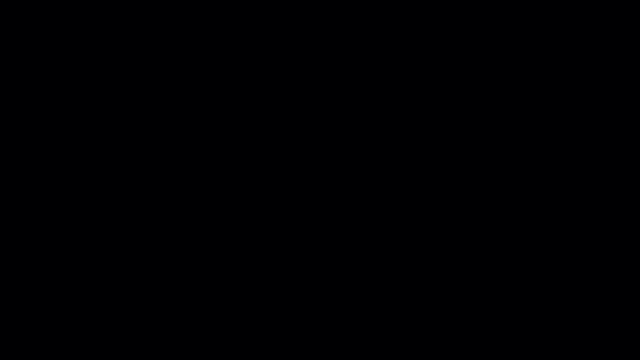 confirm it using that technique now let's work on simple multiplication problems 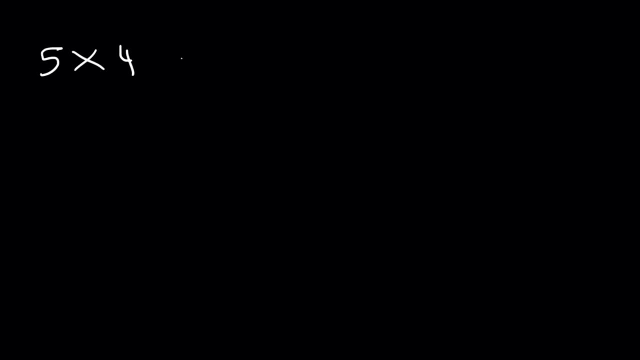 what is five times four so hopefully you've committed this memory you know your multiplication tables up to 12 but let's say if you don't know it what is five times four five times four is basically five added four times 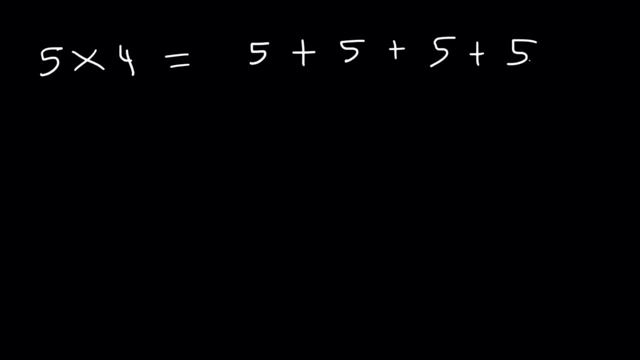 multiplication what it really is is repeat addition so five times four means you're adding five four times five plus five is 10 the other two fives add up to 10 10 plus 10 is 20 so five times four is 20 you could also see it this way five times four and four times five are the same four times five means that you're adding four five times four plus four is eight the next two fours add up to eight and then we have one four 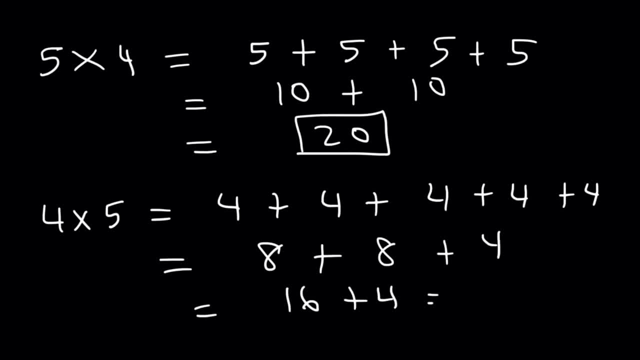 remaining eight plus eight is sixteen sixteen plus four is twenty so you get the same answer so let's say if we want to find the value of six 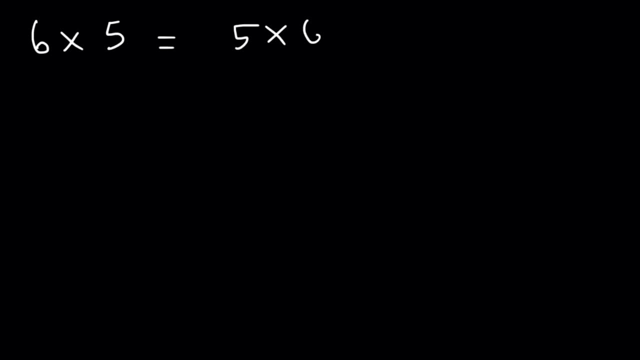 times five which is the same as five times six all we need to do is add six five times or add five six times which have is easier six plus six is 12 so these two add up to 12 as well and 12 plus 12 is 24 plus six that's 30 so six times five or five times six 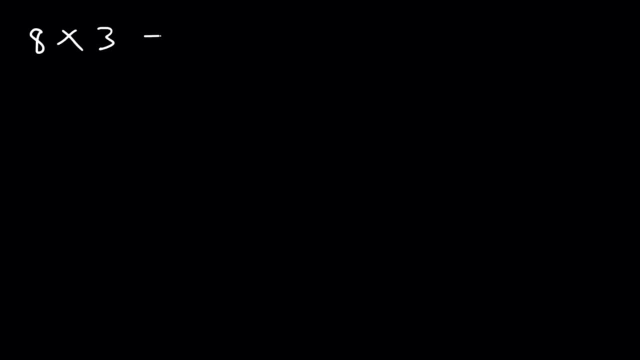 is 30 now what about eight times three this is simply 8 plus 8 plus 8 three times 8 plus 8 is 16 and what's 16 plus 8 well 6 plus 8 is 14 so think of 16 as 10 plus 6 plus 8 and if 6 plus 8 is 14 and 10 plus 14 is 24 then 8 times 3 is 24 now what about this example 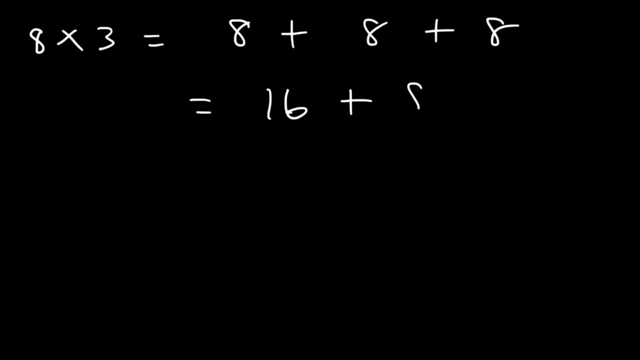 three times 8 plus 8 is 16.. And what's 16 plus 8?? Well, 6 plus 8 is 14.. So think of 16 as 10 plus 6 plus 8.. And if 6 plus 8 is 14, and 10 plus 14 is 24,, then 8 times 3 is 24.. 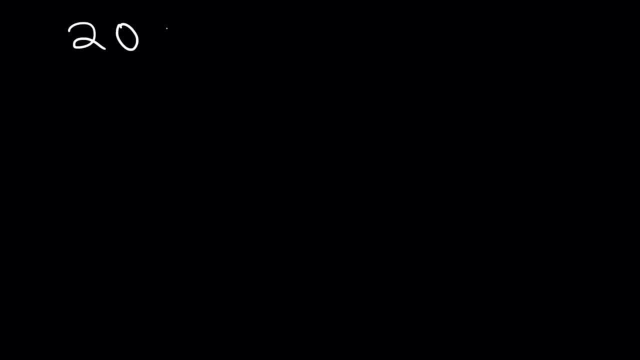 Now, what about this example? Let's use two digit numbers instead. What's 20 times 13?? Now, sometimes it might be useful to think of math in terms of money. So imagine if you have 13 $20 bills. What is the value of 13 $20 bills? Well, you know, the value of 5: 20s is 100.. Another set of 5 20s is: 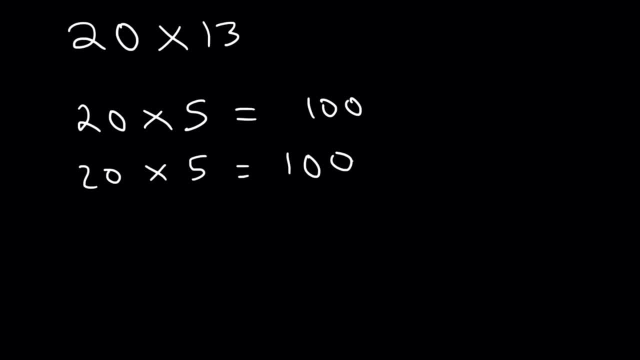 another 100.. So that's 10 20s you have. So you have three 20s left over. Three 20s is 60.. So at this point you've added 13 20s. 5 plus 5 plus 3 is 13.. So if you add a 100 plus 100 plus 60,. 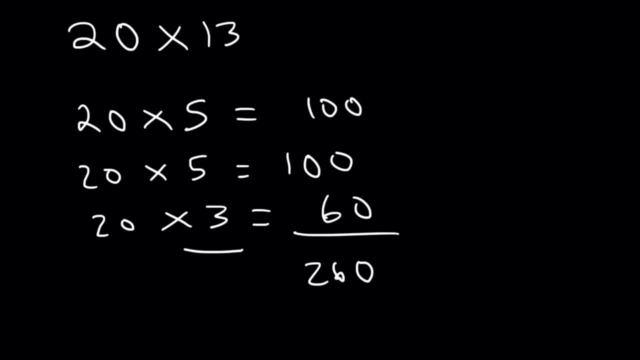 you have 260.. So 13- 20s equate to $260.. Another way in which you can get that same answer is you can break down 13 into 10 plus 3, and then use the distributive property. 20 times 10 is 200,. 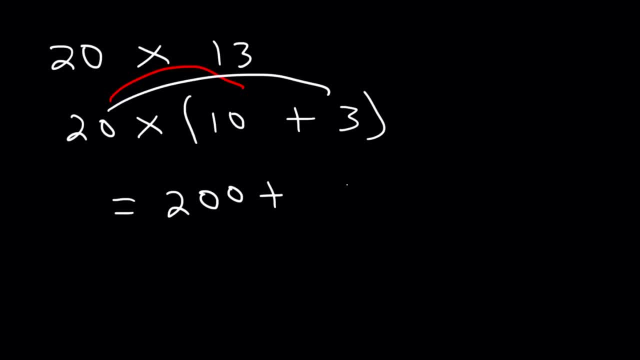 and 20 times 3 is 60. So 200 plus 60 gives you 260.. So that's another way you can do it. Let's try another example. What is 25 times 7?? So imagine if you have 7 quarters, What is the value of 7? 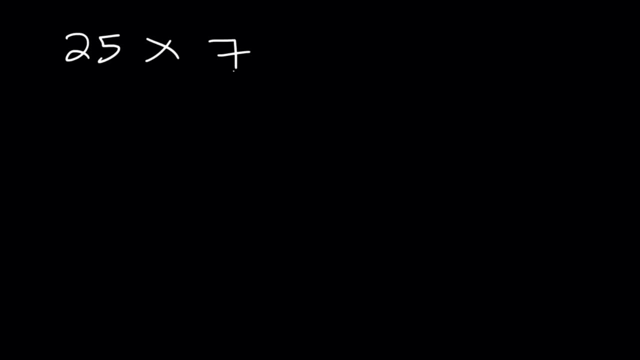 quarters. 7 quarters is $1.75.. Therefore, 25 times 7 is 175.. Now let's confirm it: 25, we could break it down into 20 plus 5.. And now let's multiply it by 7.. So what is 7 times 20?? Well, we know: 7, $20. 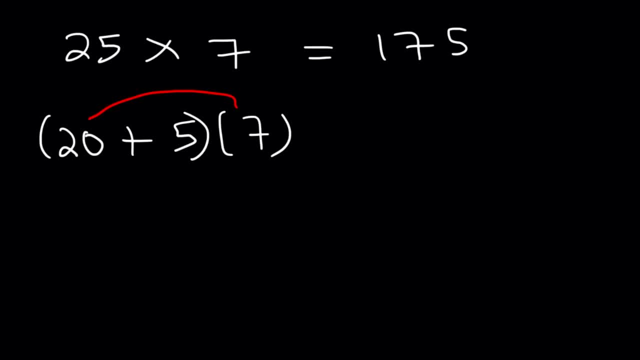 bills is $140.. And 7 times 2 is 14.. If you add the 0, you're going to get 140., And then 7 times 5 is 35. So now, if you want to add 140 plus 35, you could break it down like this: 35 is 30 plus 5.. 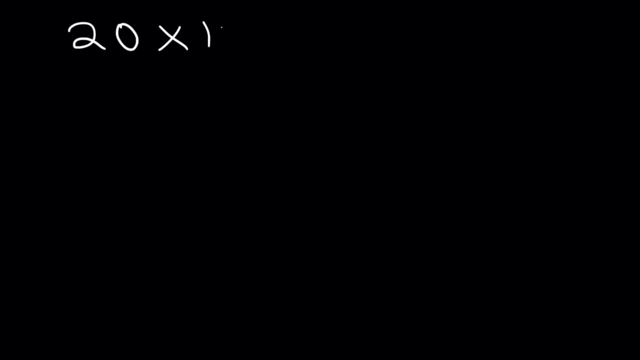 let's use two digit numbers instead what's 20 times 13 now sometimes it might be useful to think of math in terms of money so imagine if you have thirteen twenty dollar bills what is the value of thirteen twenty dollar bills 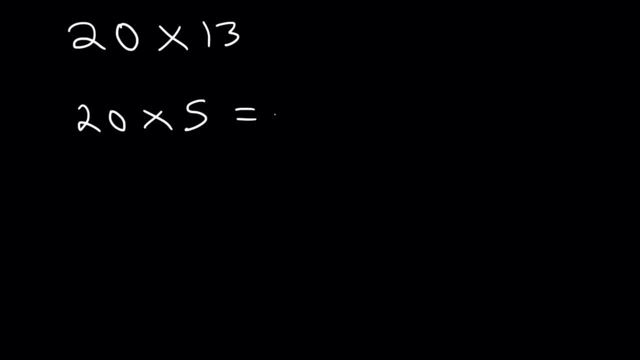 well you know the value of 520s is a hundred another set of 520s is another 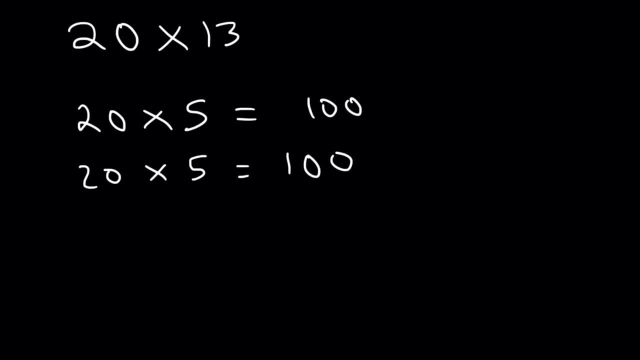 hundred so that's 1020s you have so you have 320s left over 320s is 60 so at this point you've added 1320s 5 plus 5 plus 3 is 13 so if you add a hundred plus a hundred plus 60 you have 260 so 1320s equate to two hundred and sixty dollars 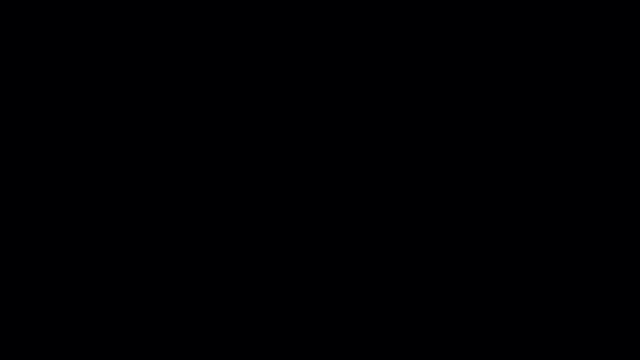 another way in which you can get that same answer is you can break down 13 into 10 plus 3 and then use the distributive property 20 times 10 is 200 and 20 times 3 is 60 so 200 plus 60 gives you 260 so that's another way you can do it 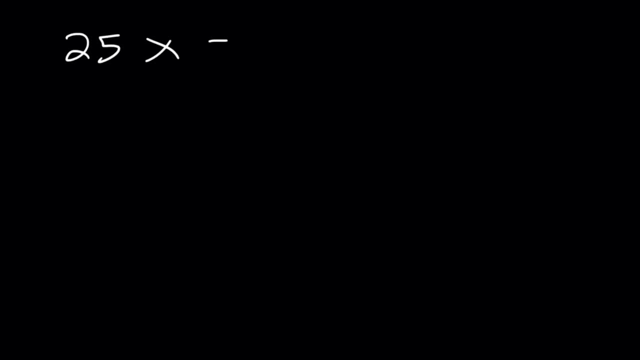 let's try another example what is 25 times 7 so imagine if you have seven 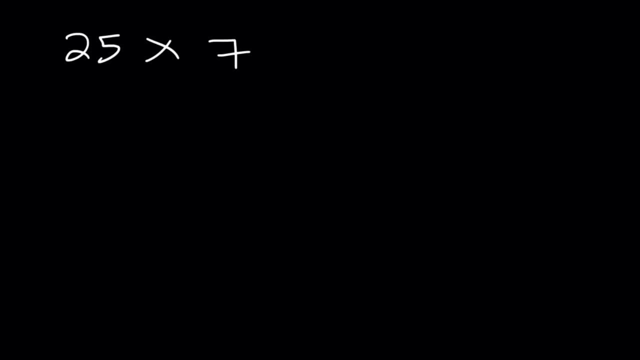 quarters what is the value of seven quarters seven quarters is a buck seventy-five therefore 25 times seven is 175 now let's confirm it 25 we could break it 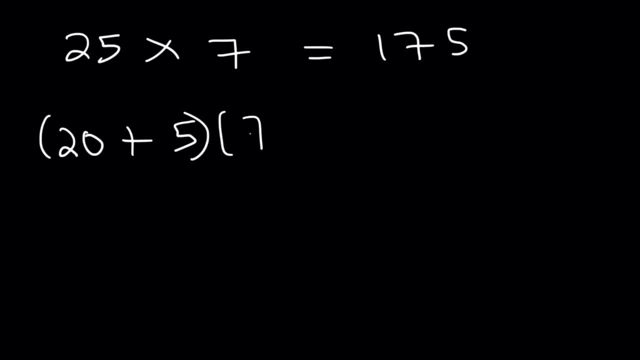 down into 20 plus five and now let's multiply it by seven so what is seven times 20 well we know 720 dollar bills is a hundred forty dollars and seven times two is 14 if you add the zero you're going to get 140 and 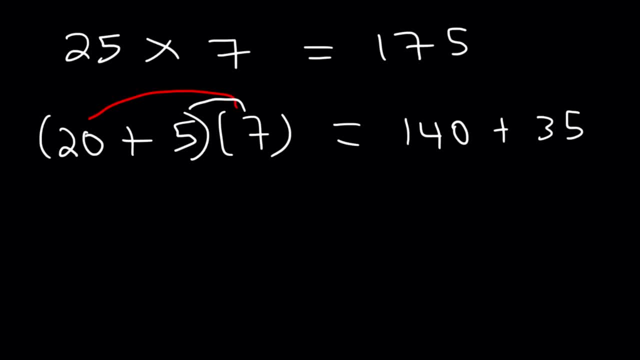 then seven times five is thirty-five so now if you want to add one 40 plus 35 you could break it down like this 35 is 30 plus 5 140 plus 30 is 170 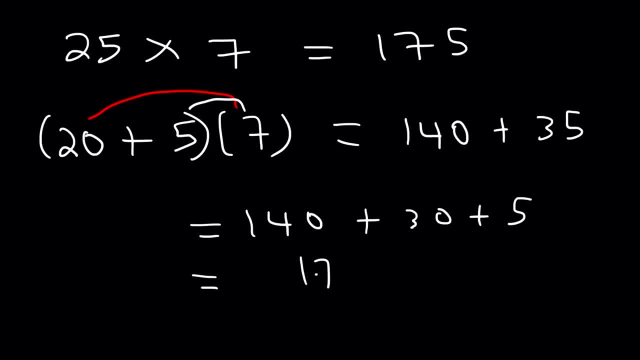 140 plus 30 is 170.. And then add 5, you get 175.. Now what is 50 times 49?? In this problem you don't want to find the value of 49 $50 bills. That's going to take some time to add that up Instead. 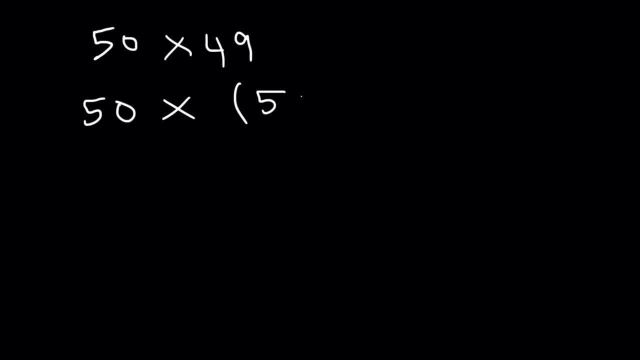 what we want to do is replace 49 with 50 minus 1.. And then distribute 50 times 50, how much is that? Well, we know, 5 times 5 is 25.. All we get to do is add the two zeros. So 50 times 50 is 2,500.. And then 50 times. 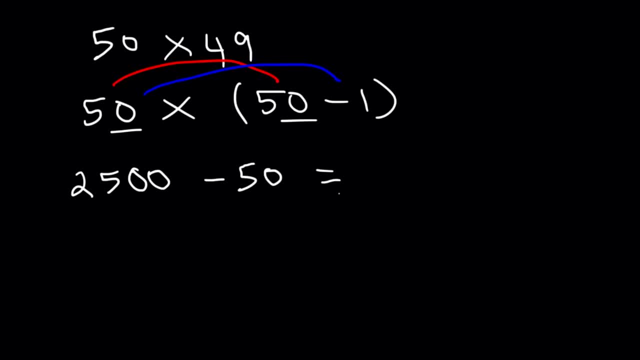 negative 1, that's negative 50. So 2,500 minus 50 is 2,450.. If you don't see this answer immediately, you could break down 2,500 into 2,400 plus 100. And you know 100 minus 50 is 50. So therefore, you're going to have 2,400 plus 50,. 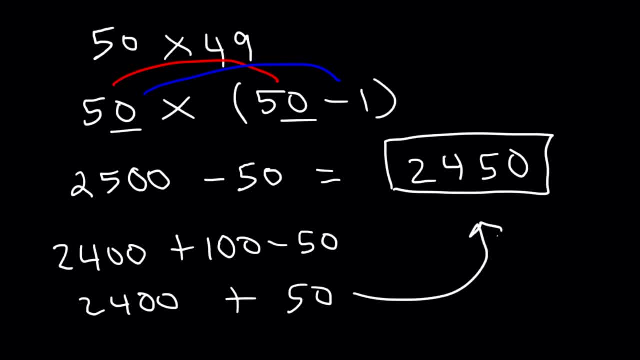 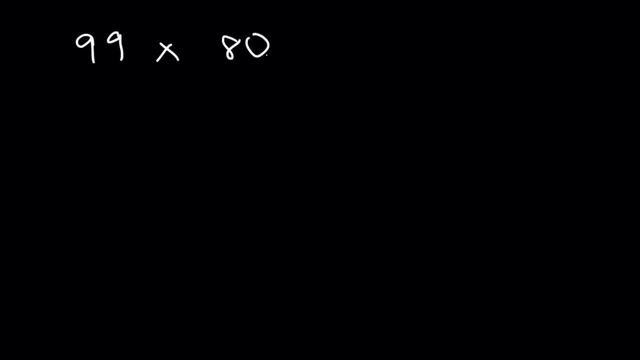 which is equal to 2,450.. So that's 50 times 49.. So what about this one? What's 99 times 80?? So, based on the last example, you know that the best way to do this is to rewrite 99 as 100 minus 1,. 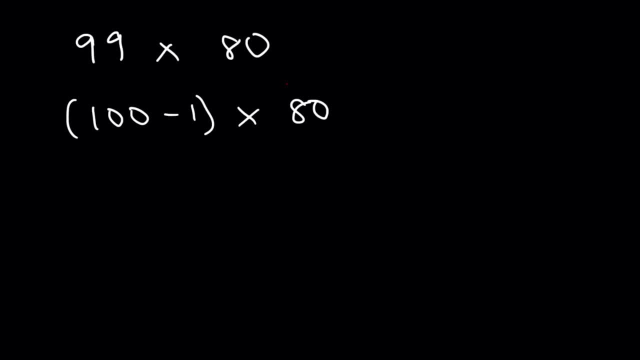 and then multiply it by 80.. So 80 times 100.. Well, 8 times 1 is 8.. And then all we got to do is add the three zeros, So this is going to be 8,000.. And then 80 times 1 is 80.. So what is 8,000 minus 80?? Well, first, 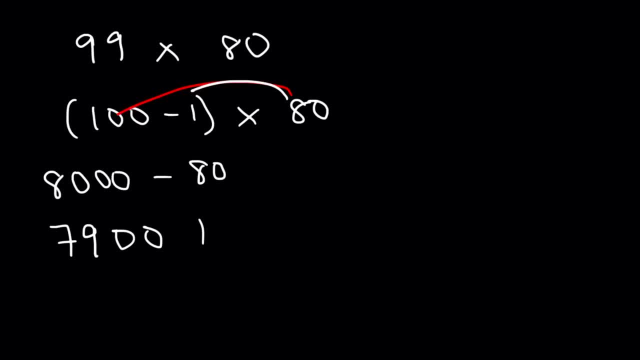 8,000 is 7,900 plus 100. And it's easy to do 100 minus 80,, that's 20. And then add 20 to 7,900. So this is going to be 7,920.. 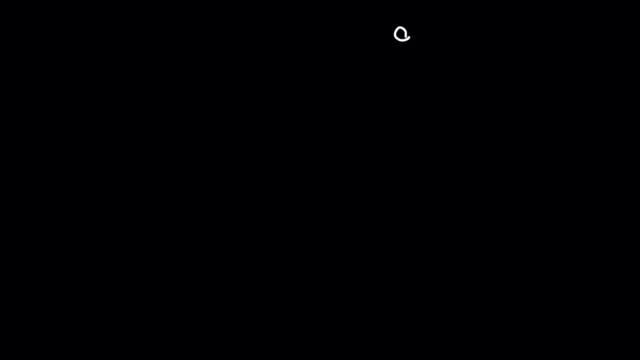 Now let's confirm this answer by using the old-fashioned multiplication technique. So 0 times 9 is 0, and that's also 0 if we multiply these two numbers. Next we need to add a 0.. 8 times 9 is 72,. carry over the 7, and then this 8 times 9 is also 72 plus 7,, that's 79.. 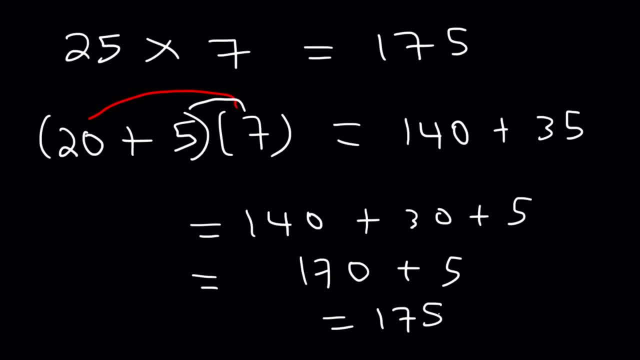 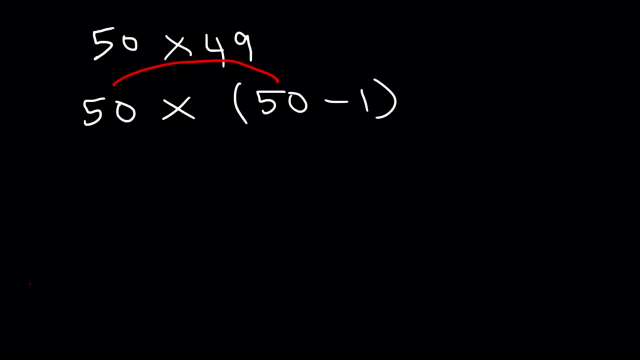 and then add five you get 175 now what is 50 times 49 and this problem you don't want to find the value of 49 50 dollar bills that's going to take some time to add that up instead what we want to do is replace 49 with 50 minus one and then distribute 50 times 50 how much is that well we know five times five is 25 all we get to do is add the two zeros so 50 times 50 is 2500 and then 50 times negative one that's negative 50 so 2500 minus 50 is 2450 if you don't see this answer immediately you could break down 2500 into 2400 plus 100 and you 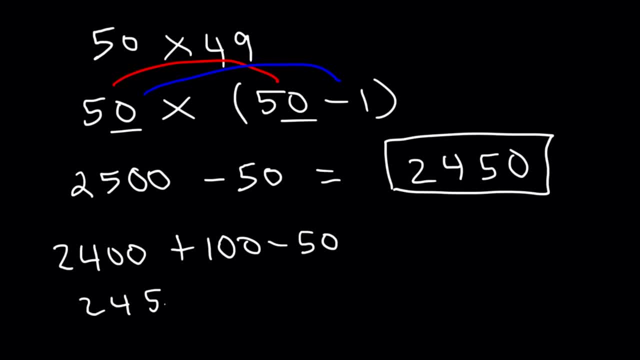 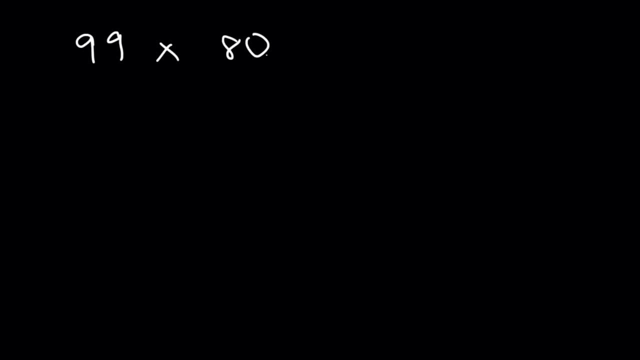 know a hundred minus 50 is 50 so therefore you can have 2400 plus 50 which is equal to 2450 so that's 50 times 49 so what about this one what's 99 times 80 so based on the last example you know that the best way to do this is to rewrite 99 as a hundred minus one and then multiply it by 80 so 80 times 100 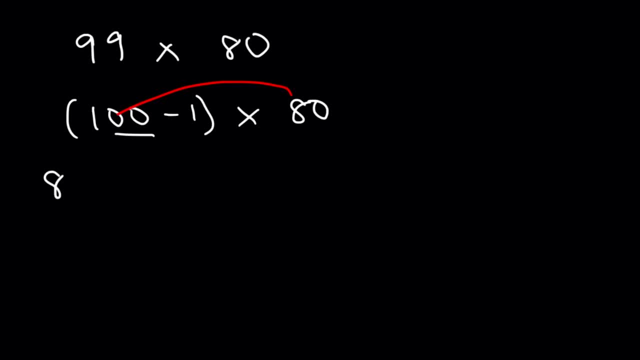 well eight times one is eight and then all we got to do is add the three zeros so this is going to be 8,000 and then 80 times one is 80 so what is 8,000 minus 80 well first 8,000 is 7900 plus 100 and it's easy to do a hundred minus 80 that's 20 and then add 20 to 7900 so this is going to be 7920 now let's confirm this answer 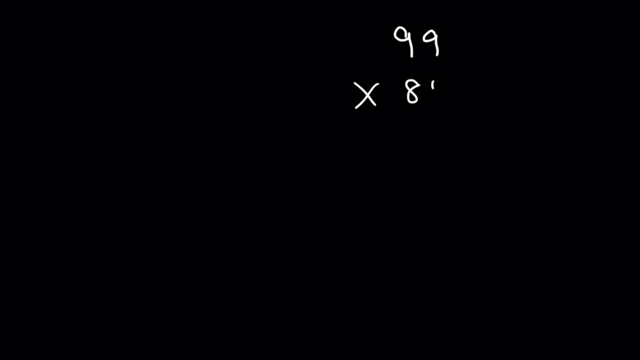 by using the old-fashioned multiplication technique so 0 times 9 is 0 and that's also 0 if we multiply these two numbers next we need to add a 0 8 times 9 is 72 carry over the 7 and then this 8 times 9 is also 72 plus 7 that's 79 so when you add this you get 7920 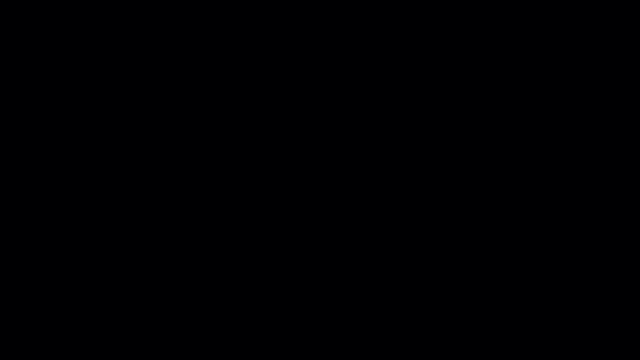 So when you add this, you get 7920.. Let's try one more multiplication example: 76 times 54.. So what I like to do is break down 76 into 70 plus 6, and 54 into 50 plus 4.. 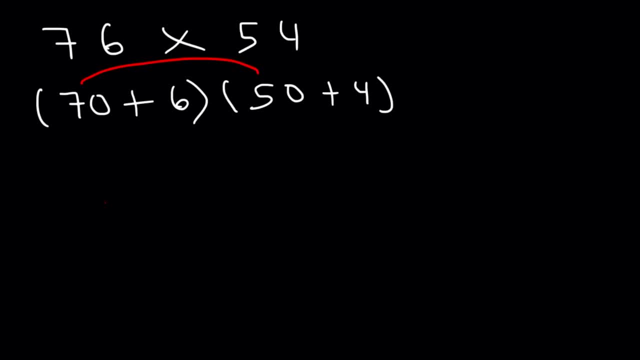 Now we need to FOIL. We need to multiply 70 times 50,. 7 times 5 is 35, and then add the two 0s. Next let's multiply 7920.. 7 times 4 is 28,, and then we just got to add one 0.. 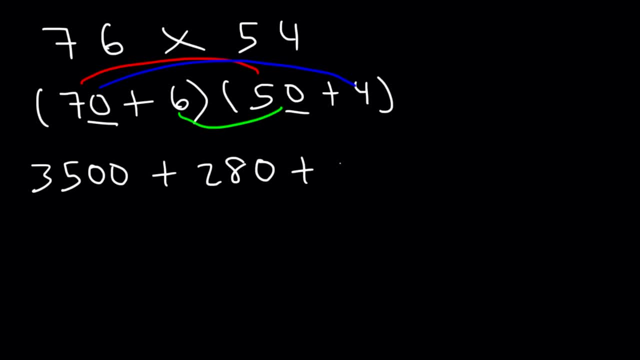 And then we have 6 times 50,. 6 times 5 is 30, and we got to add a 0, so 6 times 50 is 300.. If you have 6 $50 bills, that's $300. 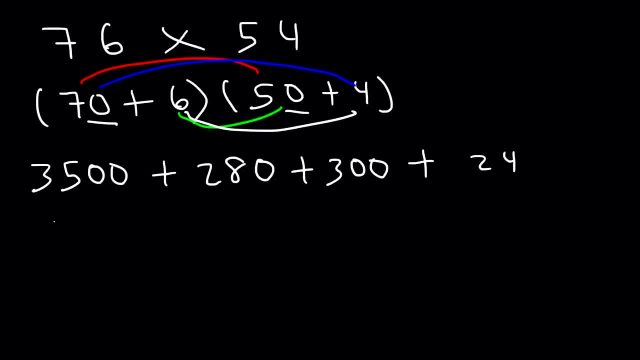 And then finally, 6 times 4 is 24.. Now we can add 300 and 280, that's going to be 580. And 24, you can think of it as 580. You can think of it as 20 plus 4.. 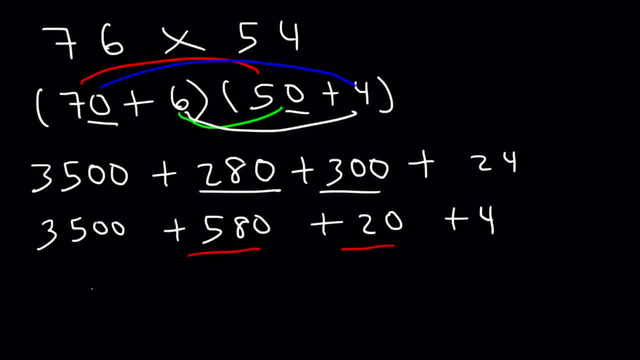 Now, 580 plus 20,, that's going to be 600.. And 3500 plus 600, well, 35 plus 6 is 41,, so this is going to be 4100.. And then plus 4, that's 4104.. 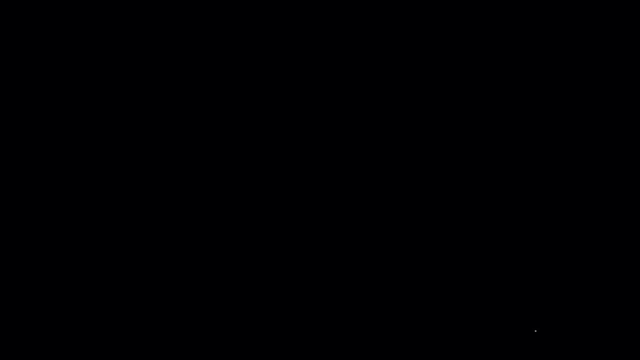 So that's how you can do it mentally. But now let's confirm that answer by multiplying these two numbers. So 6 times 4 is 24,. carry over the 2.. And then 7 times 4 is 28 plus 2, that's 30.. 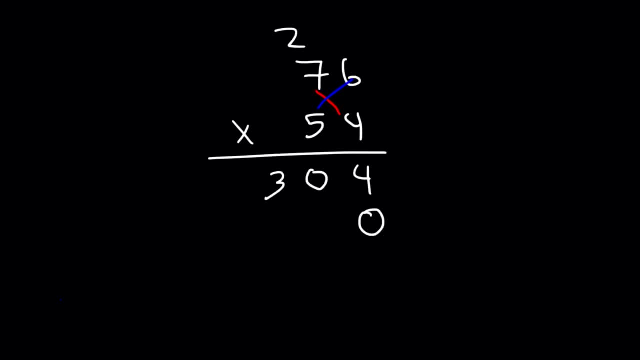 Now we need to add a 0.. 5 times 6 is 30,, so we're going to add a 3.. And then 5 times 7 is 35 plus 3,, that's 38.. Now let's add: 4 plus 0 is 4, and 0 plus 0 is 0. 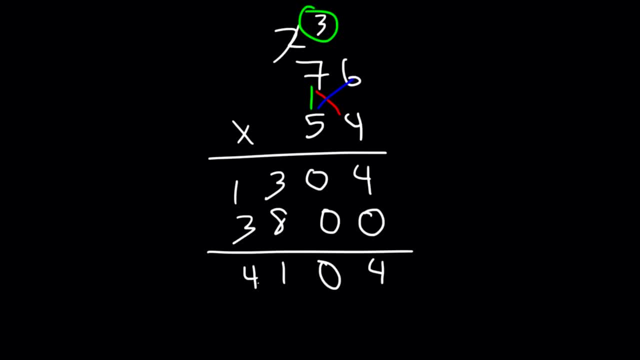 3 plus 8 is 11,. carry over the 1.. 3 plus 1 is 4.. So we get the same answer: 4104.. Now let's move on to division. So let's say if we want to divide 324 by 2.. 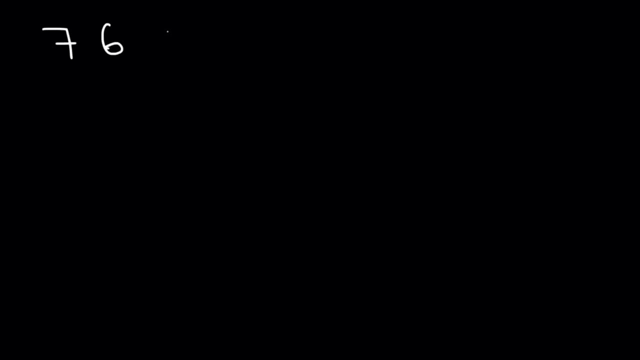 let's try one more multiplication example 76 times 54 so what I like to do is break down 76 into 70 plus 6 and 54 into 50 plus 4 now we need to FOIA we need to multiply 70 times 50 7 times 5 is 35 and then add the two zeros next let's multiply 70 times 4 7 x 4 is 20 and then we just got to add one zero and then we have 6 times 50 6 times 5 is 30 and we got to add a 0 so 6 times 50 is 300 if you have 650 dollar bills that's 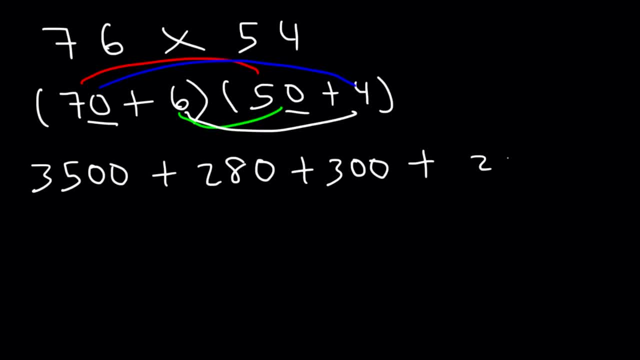 $300 and then finally 6 times 4 is 24 now we can add 300 and 280 that's going to be 580 and 24 you can think of it as 20 plus 4 now 580 plus 20 that's going to be 600 and 3500 plus 600 will 35 plus 6 is 41 so this is going to be 4100 and then plus 4 that's 4104 so that's how you can do it mentally but now let's 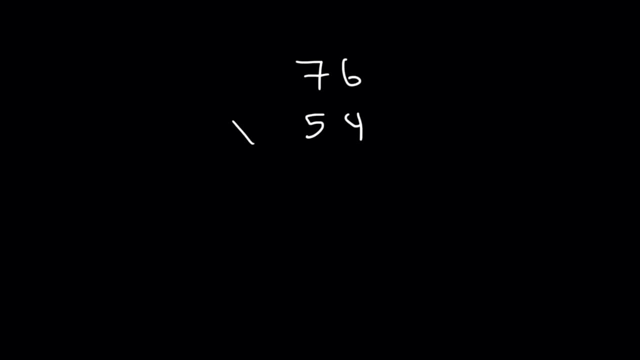 confirm that answer by multiplying these two numbers. So 6 times 4 is 24, carry over the 2, and then 7 times 4 is 28 plus 2, that's 30. Now we need to add a 0. 5 times 6 is 30, so we're going to add a 3, and then 5 times 7 is 35 plus 3, that's 38. Now let's add 4 plus 0 is 4, 0 plus 0 is 0, 3 plus 8 is 11, carry over the 1, 3 plus 1 is 4. So we get the same 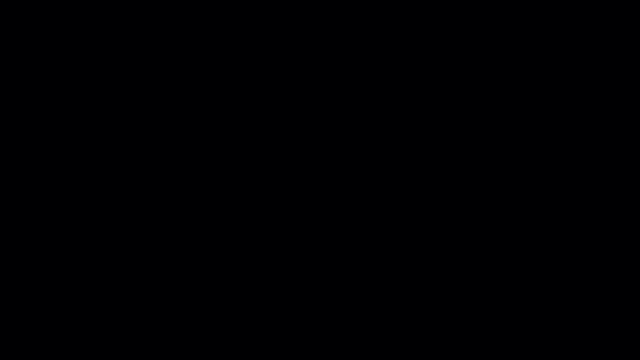 answer, 4,104. Now let's move on to division. So let's say if we want to divide 324 by 2, 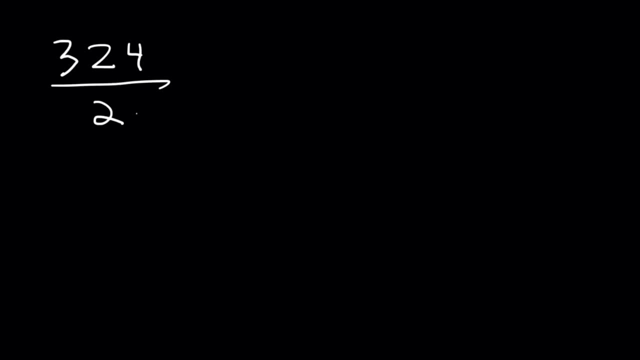 how can we do so mentally? So first, divide 32 by 2, that is equal to 16. 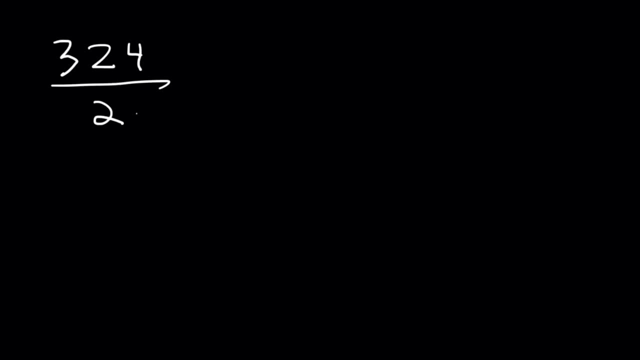 How can we do so mentally? So first divide 32 by 2.. That is equal to 16.. And then divide 4 by 2.. That's equal to 2.. So it turns out that 324 divided by 2, if you type it in your calculator- you're going to get 162. 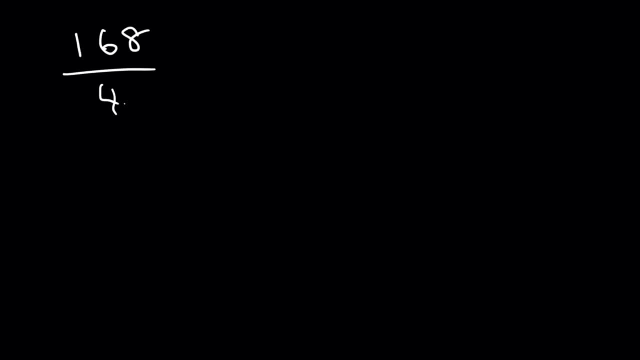 So here's another example: 168 divided by 4.. Notice that 16 and 8 are multiples of 4.. So we can use that simple division trick. So first let's divide 16 by 4.. 16 divided by 4 is 4.. 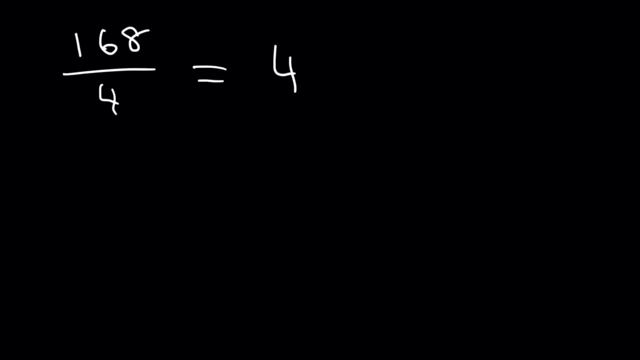 Next, let's divide 8 by 4.. 8 divided by 4 is 2.. So this will give you 42. And it's always good to confirm your answer with a calculator just to make sure you're doing it correctly. 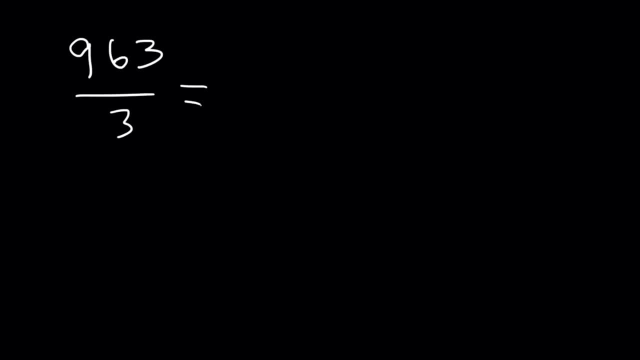 Try this one: 963 divided by 3.. Now we really don't have to do 996 divided by 3, because 9,, 6, and 3 individually are all multiples of 3.. So first let's divide 9 by 3.. 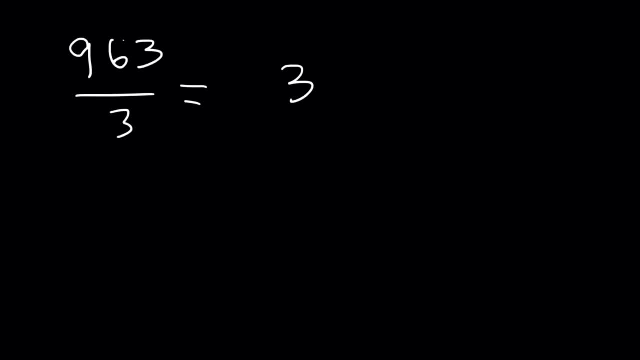 We can do it one at a time: 9 divided by 3 is 3.. 6 divided by 3 is 2.. And 3 divided by 3 is 1.. So therefore, this is 321.. Now what if we don't have a nice number? 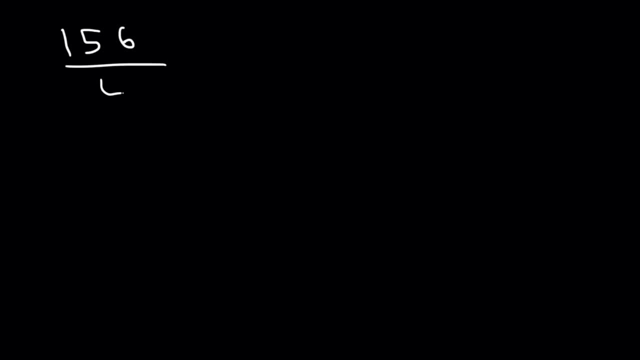 For example, let's say 156 divided by 4. 15 is not divisible by 4. And 6 is not either. So what can we do in this example, In a situation like this? break down 156 into smaller numbers, numbers that are divisible by 4.. 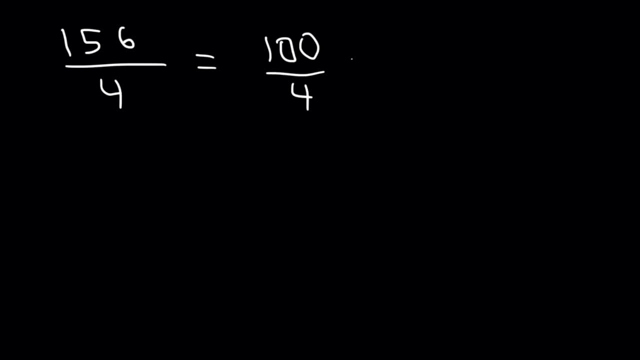 For example, 100 is divisible by 4. And 40 is divisible by 4. And 16 is divisible by 4.. 40 plus 16 is 56. And 56 plus 100 is 156.. So both sides of the equation are equivalent. 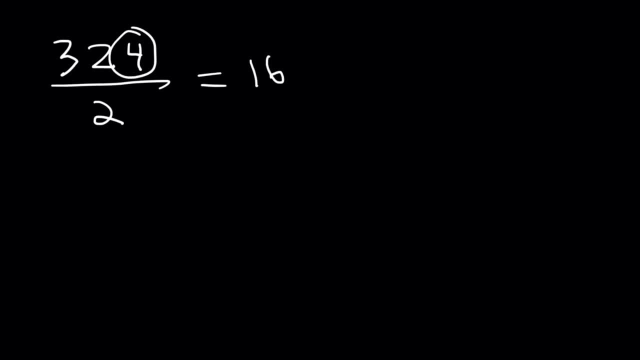 And then divide 32 by 2, that is equal to 16. And then divide 32 by 2, that is equal to 16. And then divide 32 by 2, that is equal to 16. And then divide 4 by 2, that is equal to 2. So it turns out that 324 divided by 2, if you type it in your calculator, you're going to get 162. 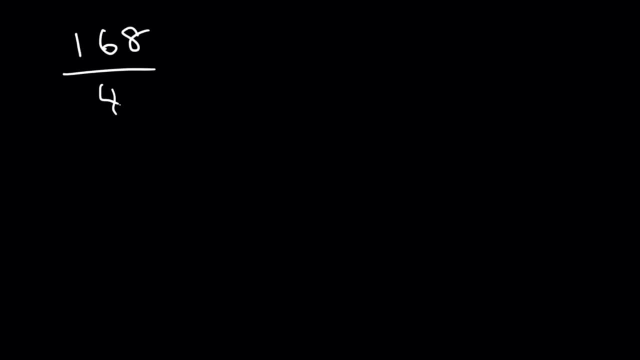 So here's another example, 168 divided by 4. Notice that 16 and 8 are multiples of 4. So we can use that simple division trick. So first, let's divide 16 by 4. 16 divided by 4 is 4. Next, let's divide 8 by 4. 8 divided by 4 is 2, so this will give you 42. 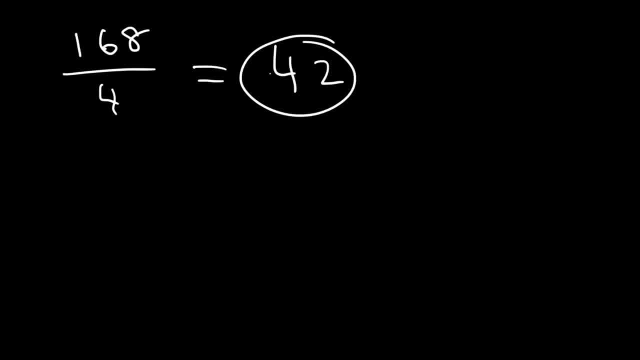 And it's always good to confirm your answer with a calculator, just to make sure you're doing it correctly. 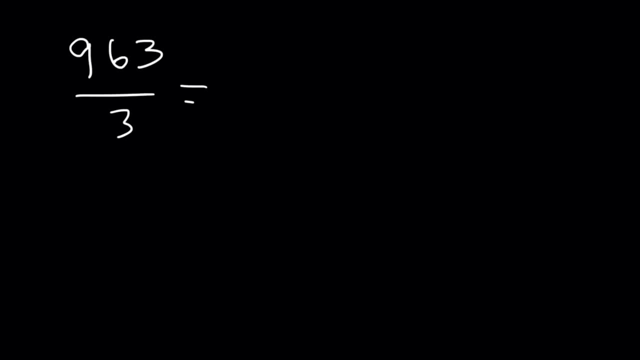 Try this one, 963 divided by 3. Now, we really don't have to do 996 divided by 3, because 9, 6, and 3 individually are all multiples of 3. 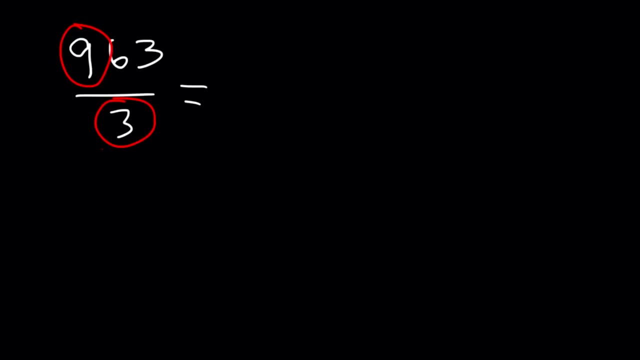 So, first, let's divide 9 by 3. We can do it one at a time. 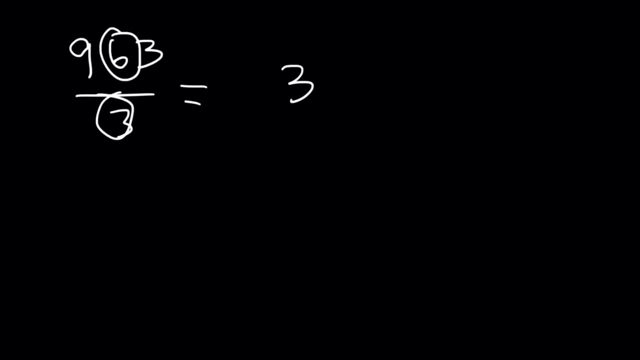 9 divided by 3 is 3, 6 divided by 3 is 2, and 3 divided by 3 is 1. So, therefore, this is 321. 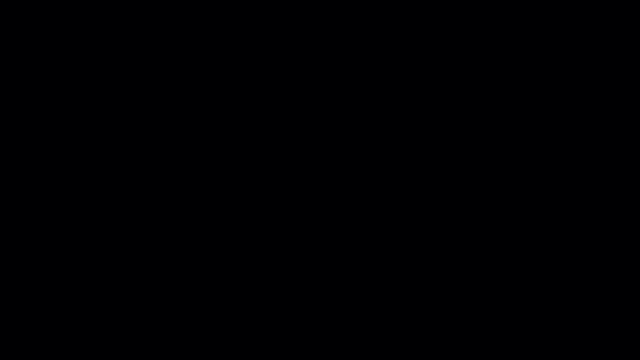 Now, what if we don't have a nice number? For example, let's say 156 divided by 4. 15 is not divisible by 4, and 6 is not either. So, what can we do in this example? 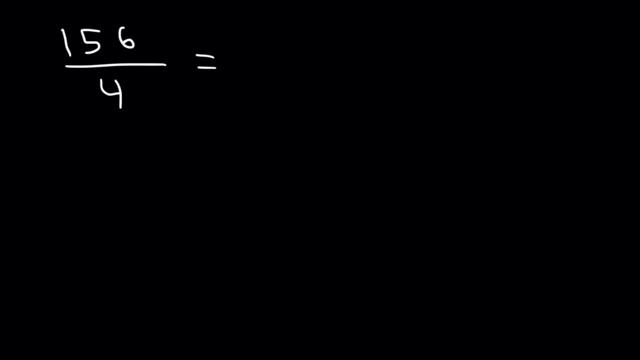 In a situation like this, break down 156 into smaller numbers, numbers that are divisible by 4. For example, 100 is divisible by 4, and 40 is divisible by 4, and 16 is divisible by 4. 40 plus 16 is 56. And 56 plus 100 is 156. So, both sides of the equation are equivalent, they're balanced, they have the same value. Now, how many times does 4 go into 100? You know 4 quarters is a dollar, so 100 divided by 4 is 25. 40 divided by 4 is 10. 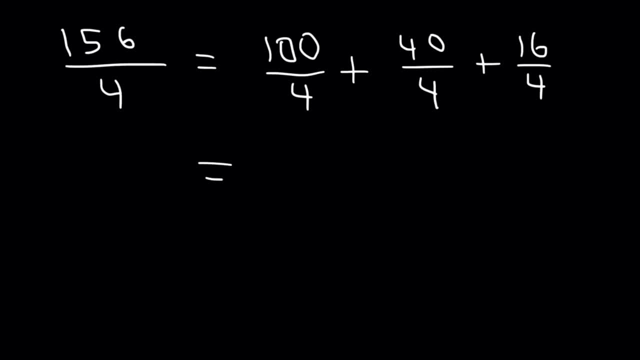 They're balanced, They have the same value. Now, how many times does 4 go into 100?? You know, 4 quarters is a dollar. So 100 divided by 4 is 25.. 40 divided by 4 is 10.. 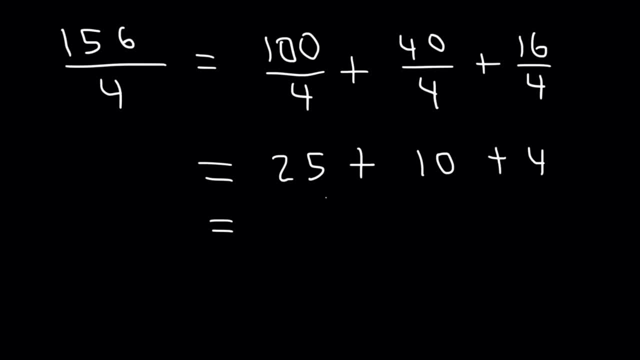 16 divided by 4 is 4.. Now, 25 plus 10 is 35.. 35 plus 4 is 39. So therefore, 156 divided by 4 is 39.. Now you can confirm it. 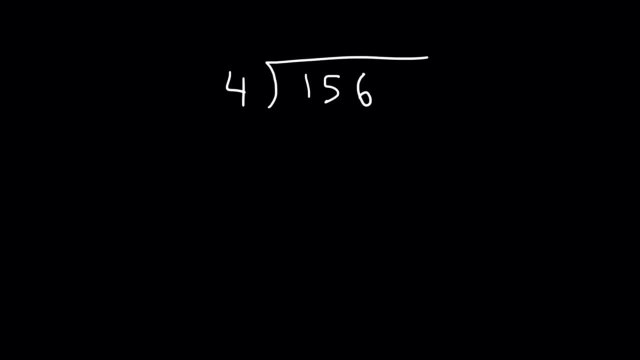 Using long division, 4 goes into 15 three times 4 times 3 is 12.. 15 minus 12 is 3.. Bring down the 6. 4 goes into 36 nine times, And so the remainder is 0.. 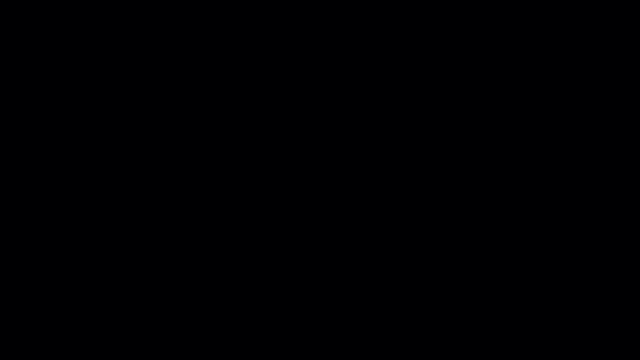 So 156 divided by 4 is 39. Now let's work on some more practice examples. Let's divide 234 by 3.. So now you don't want to use 200.. 200.. 200 is not a multiple of 3.. 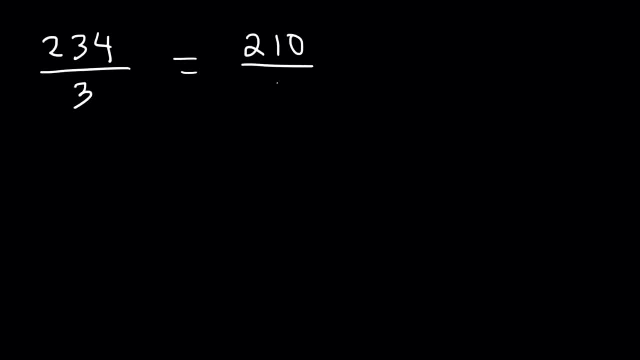 However, you can use 210, because 3 goes into 21.. So 3 will go into 210.. And you also could use 24, because 24 is a multiple of 3. So you want to break down 234 into 210 and 24.. 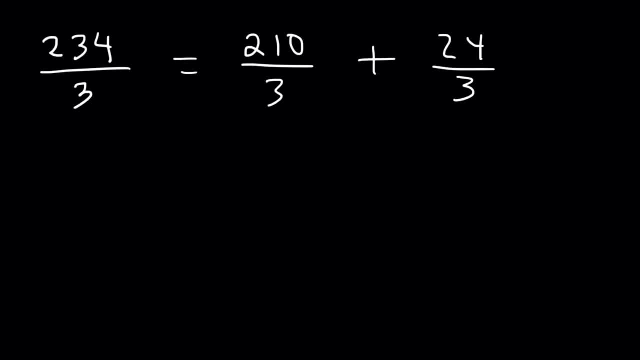 You want to break it down into two numbers that are both divisible by 3.. Now we know that 21 divided by 3 is 7.. So 210 divided by 3 is 70. And 24 divided by 3 is 7.. 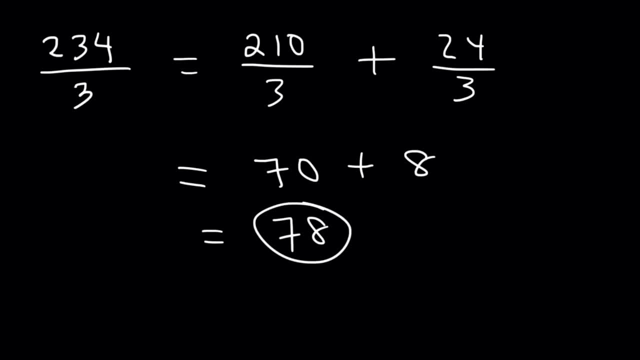 So 24 divided by 3 is 8.. So this is equal to 78.. Now let's confirm it. using long division, 3 goes into 23. seven times 3 times 7 is 21.. 23 minus 21 is 2.. 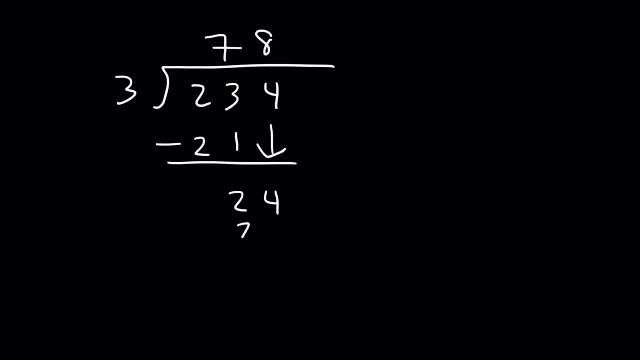 Bring down the 4.. 3 times 8 is 24.. So, as you can see, this is equal to 78.. Let's try another example: 84 divided by 7.. So what two numbers should we break down 84 into? 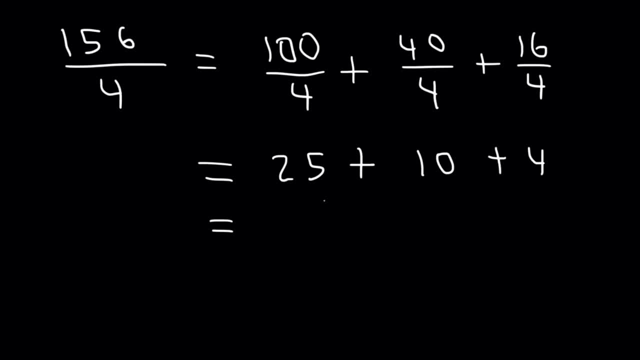 16 divided by 4 is 4. Now, 25 plus 10 is 35. 35 plus 4 is 39. So, therefore, 156 divided by 4 is 39. 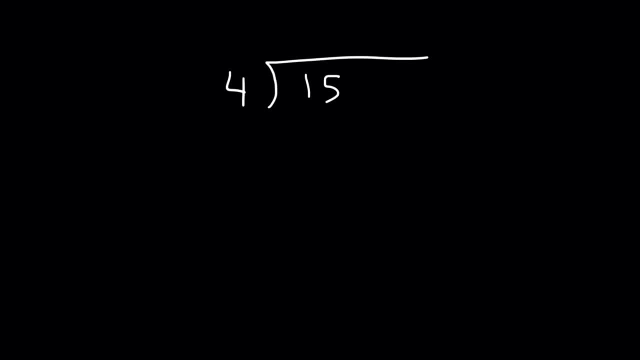 Now, you can confirm it using long division. 4 goes into 15 three times. 4 times 3 is 12. 15 minus 12 is 3, bring down the 6. 4 goes into 36 nine times, and so the remainder is 0. So, 156 divided by 4 is 39. Now, let's work on some more practice examples. 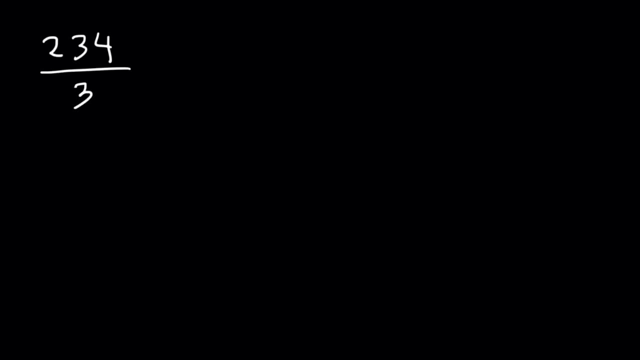 Let's divide 234 by 3. So, now, you don't want to use 200. 200 is not a multiple of 3. However, you can use 210. Because 3 goes into 21, so 3 will go into 210. And you also could use 24, because 24 is a multiple of 3. So, you want to break down 234 into 210 and 24. 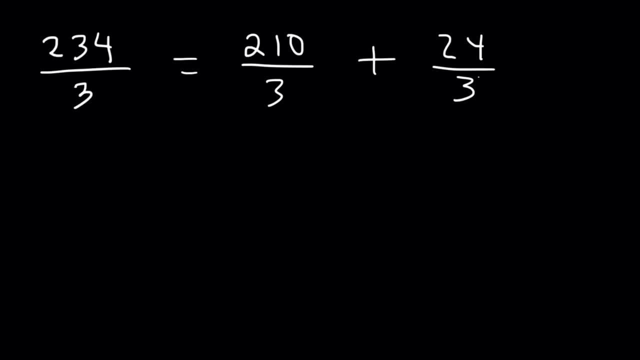 You want to break it down into two numbers that are both divisible by 3. Now, let's look at the next example. So, you want to break down 234 into 210 and 24. You want to break it down into two numbers that are both divisible by 3. 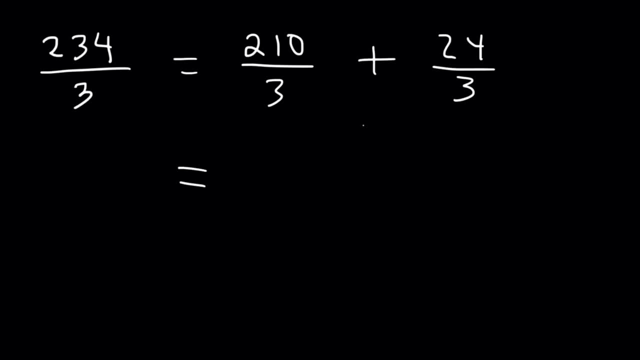 Now, we know that 21 divided by 3 is 7. So, 210 divided by 3 is 70. And 24 divided by 3 is 8. So, this is equal to 78. 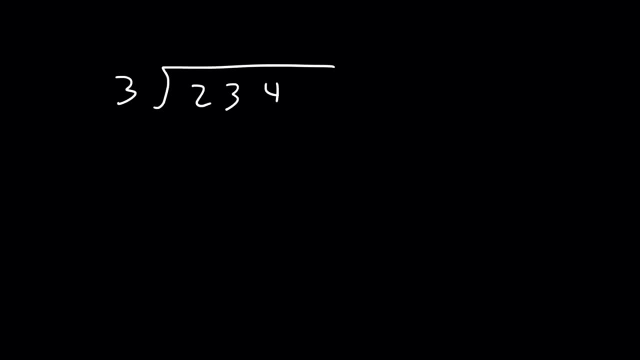 Now, let's confirm it using long division. 3 goes into 23 seven times. 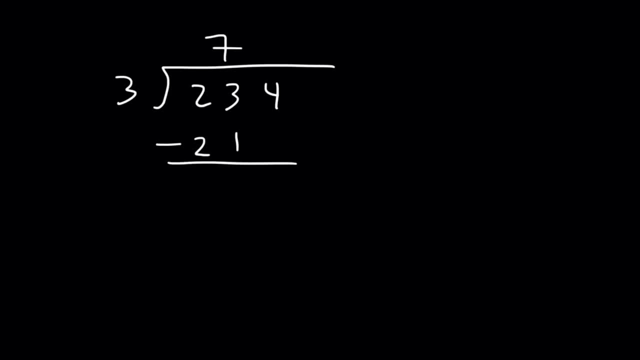 3 times 7 is 21. 23 minus 21 is 2. Bring down the 4. 3 times 8 is 24. So, as you can see, this is equal to 78. 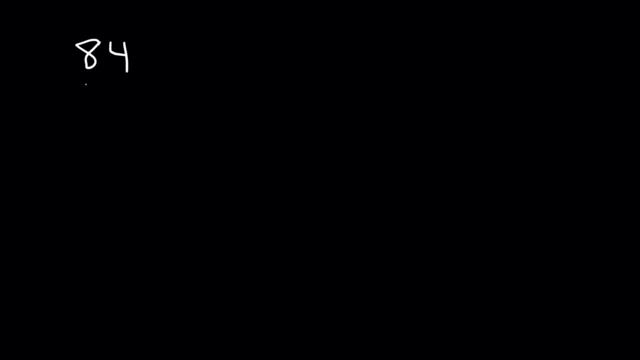 Let's try another example. 84 divided by 7. So, what two numbers should we break down 84 into? What I would choose is 70 and 14. 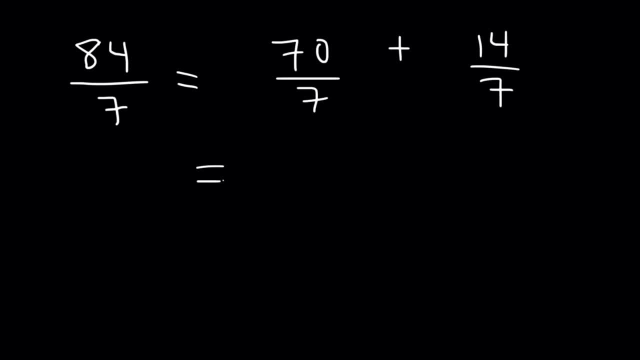 Because they're both divisible by 7. 70 divided by 7 is 10. 14 divided by 7 is 2. 10 plus 2 is 12. So, 84 divided by 7 is 12. 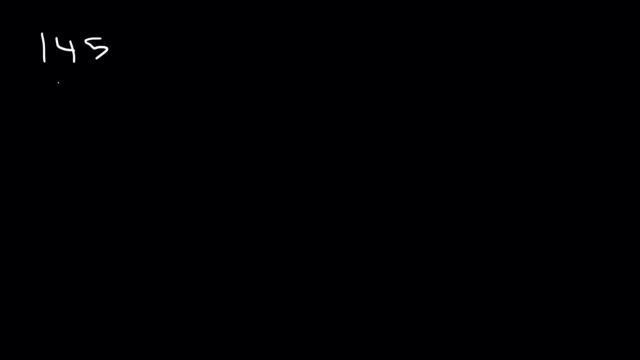 Now, what about 145 divided by 5? Now, what about 145 divided by 5? So, what would you do?